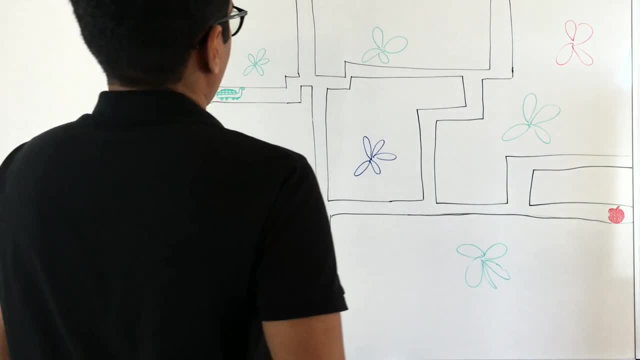 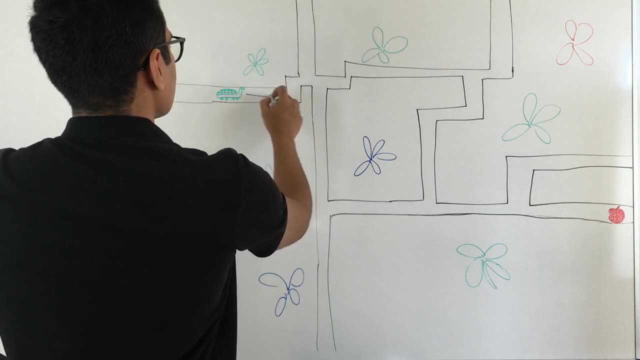 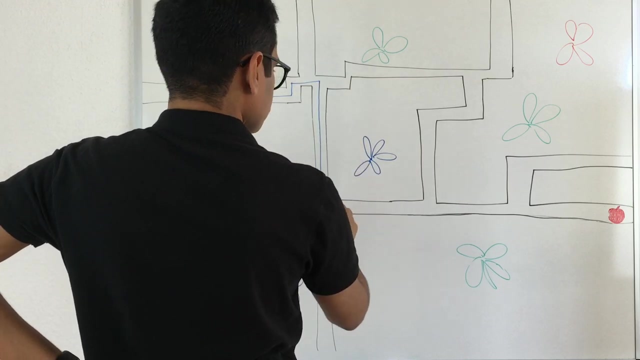 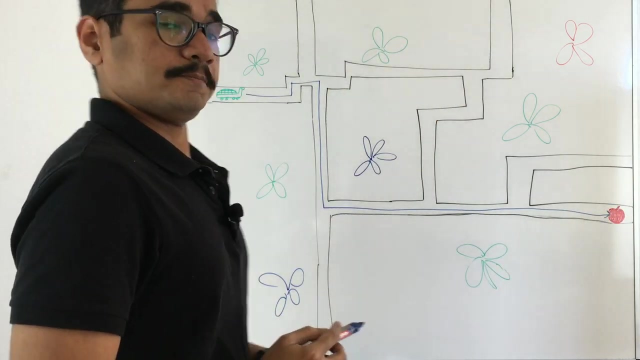 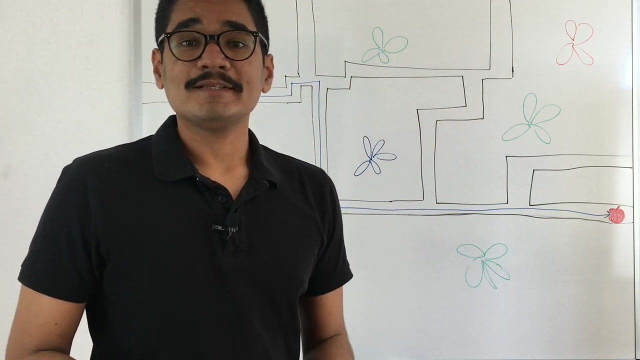 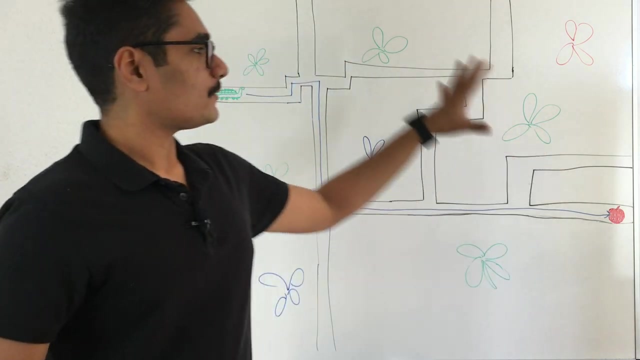 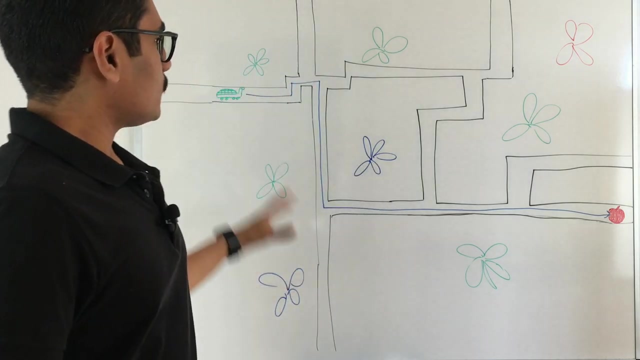 Oh hi, I am very fond of solving this kind of simple kids problem, So that's my weakness. So whenever in childhood I saw some kind of this maze problem, It used to very much amuse me a lot. So essentially in machine learning we have these kind of steps that is going around, So that mainly 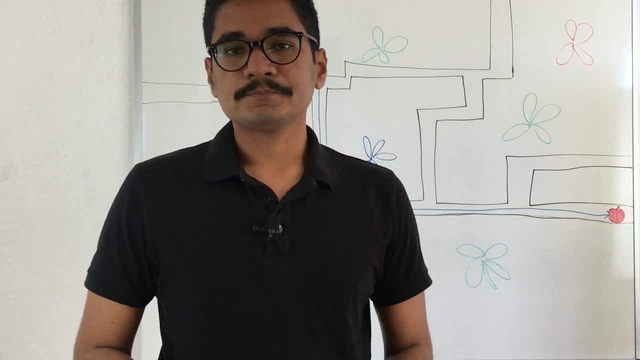 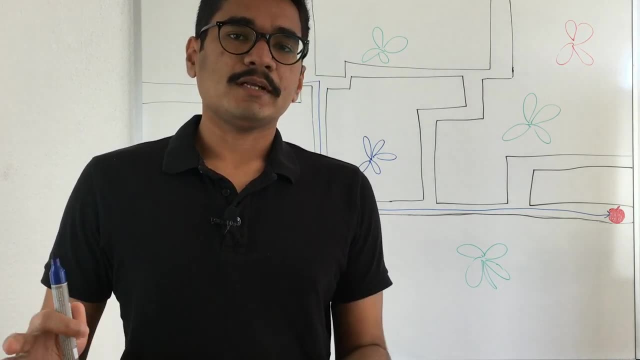 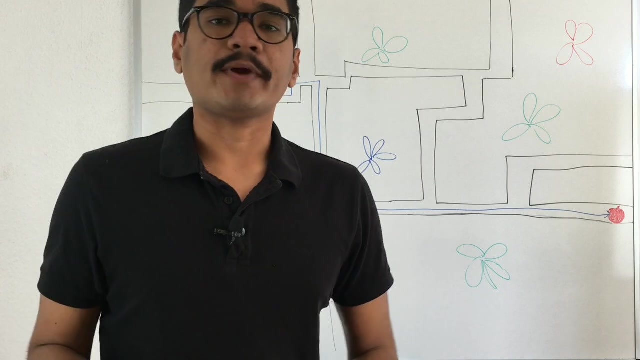 is in the reinforcement learning or for game development. So an agent will learn how to pick up the paths. So when we were kids or at the lower level, we used to solve this kind of small, small maze problem in order to find the path, and there was some constraint. 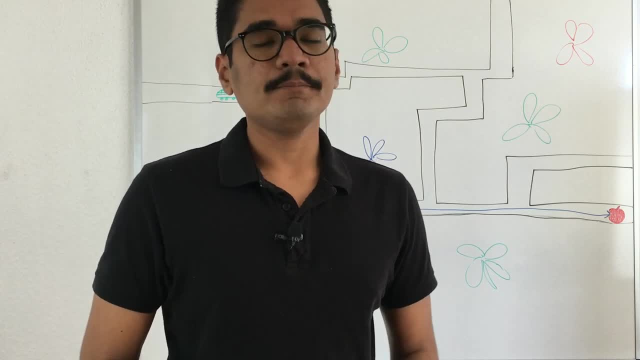 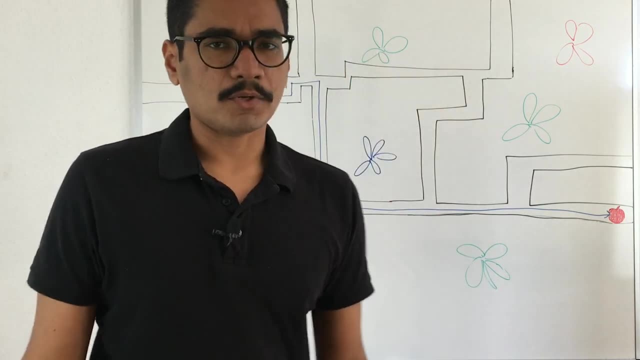 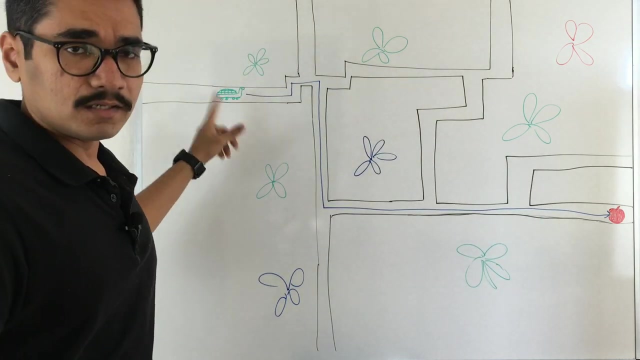 like, we want to find the path in minimal, optimal time, which is possible, and we want to maximize the reward. So this is a very simple maze problem that you see. So here you don't see any constraint as such, Just the agent. here You can see a turtle and here there is a fruit. So that is the 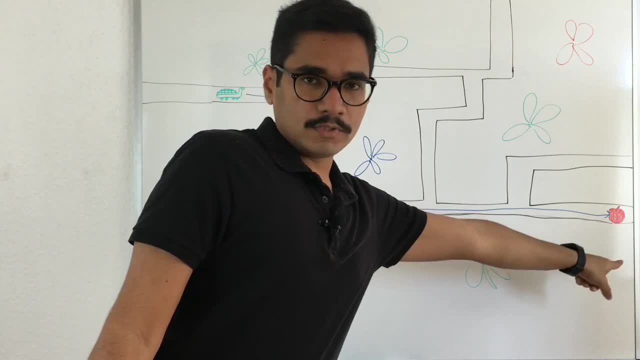 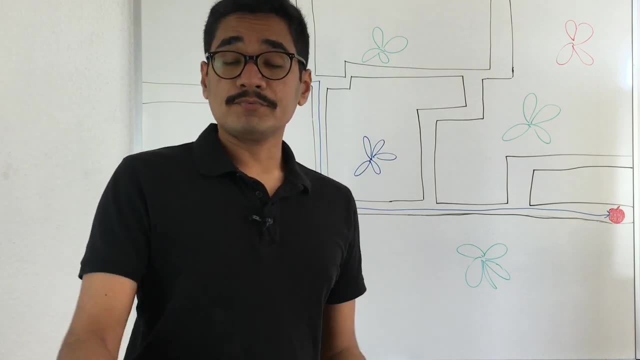 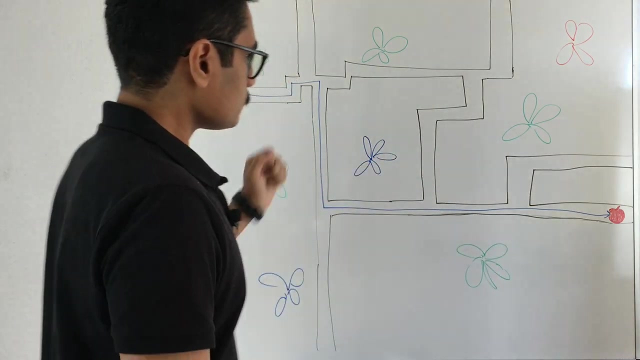 reward, and there are not many rewards, just only one reward. Also, there are no constraints, but in the real world, when you have played different games, there will be different kinds of constraints that will be put forth in front of you when you solve this kind of problems. 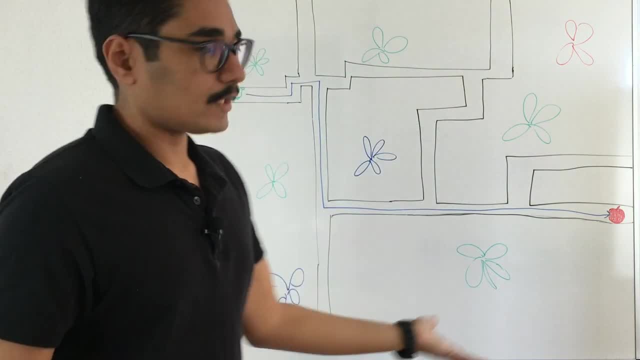 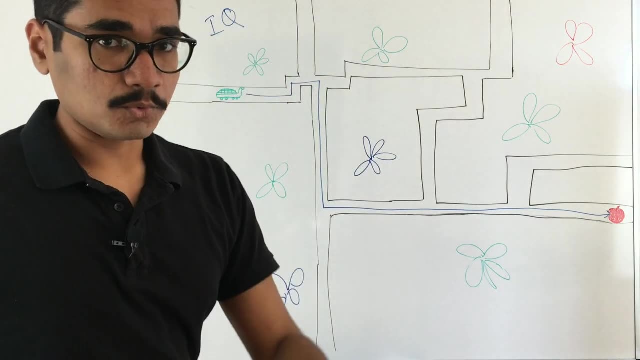 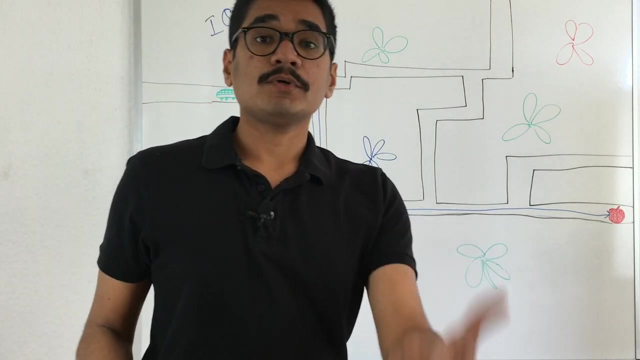 So when, as a child, we used to solve this kind of problems, it was basically in order to improve our IQ or test our IQ. that is, intelligent quotient. So this particular kind of maze problem or this kind of learning where we want to find the optimal path in reinforcement. 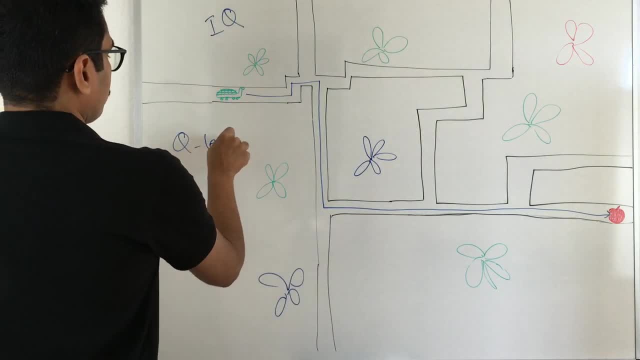 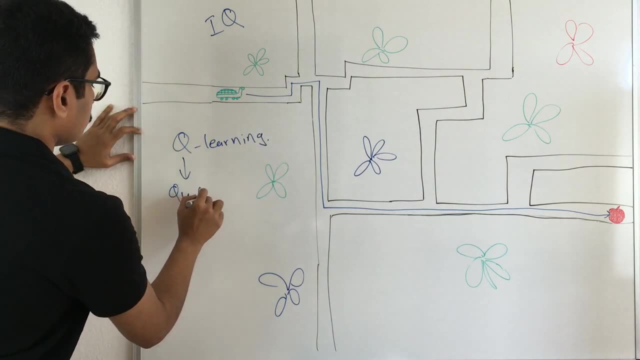 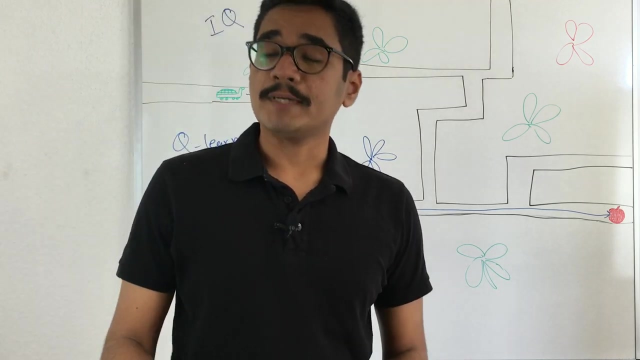 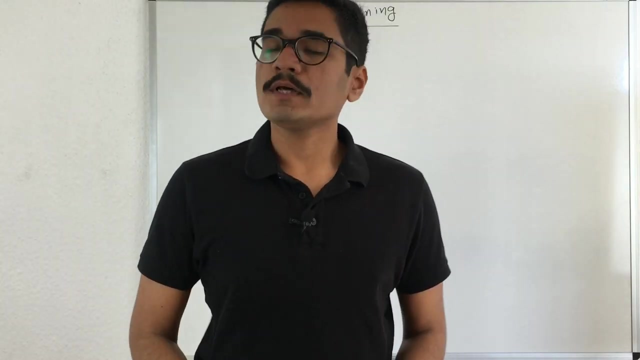 learning is called as Q learning, So the Q in Q learning stands for quality, And so the topic Video is Q learning, and we'll see what are the mathematics behind Q learning. So let's get started, Okay, So before we begin about the Q learning algorithm, we have to understand. 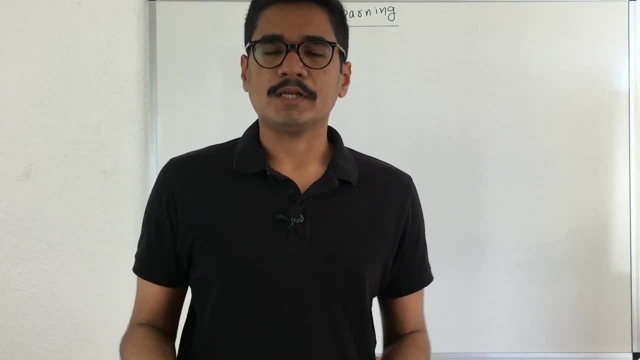 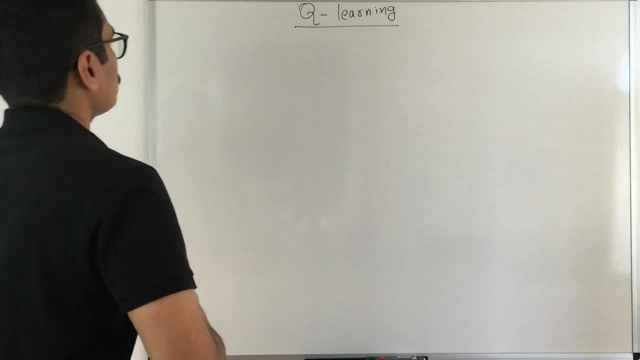 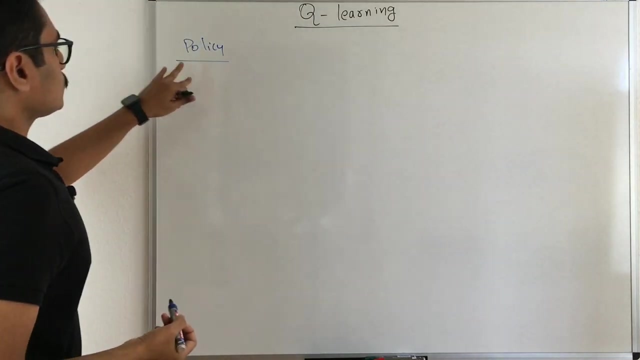 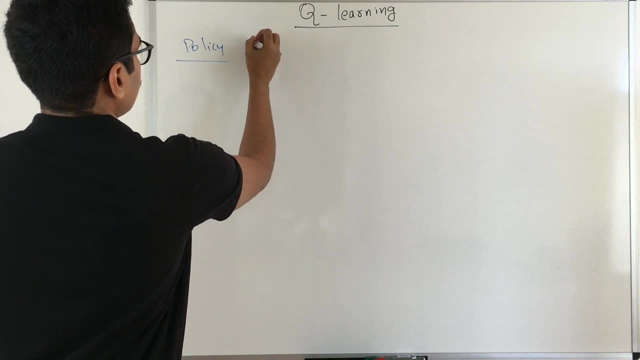 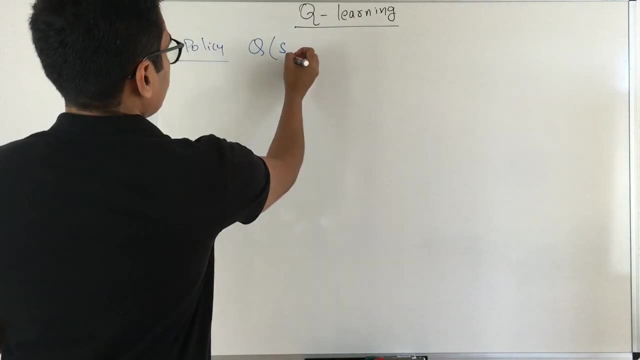 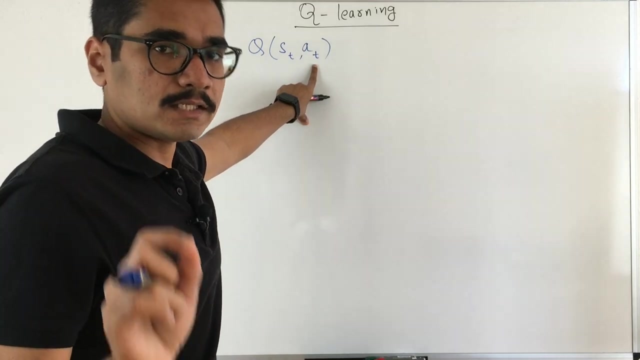 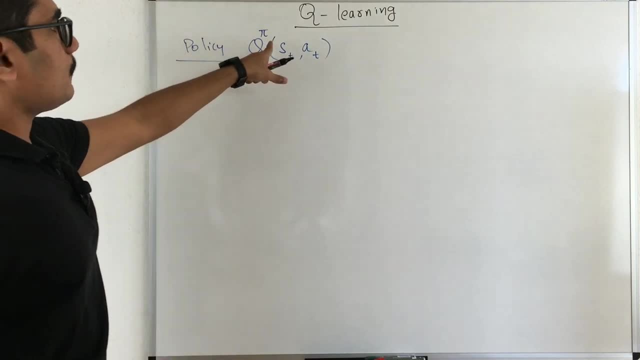 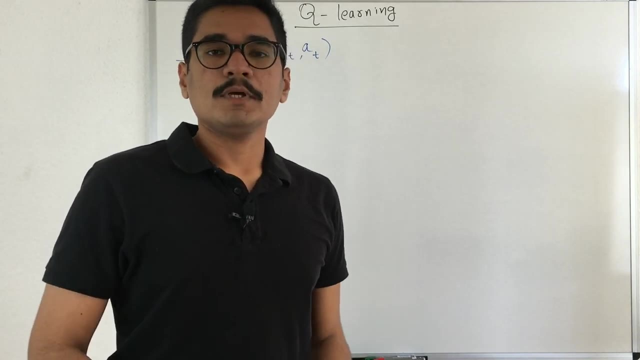 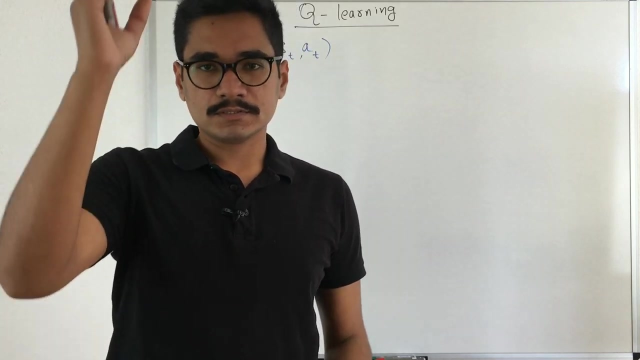 So, So, given by a pie on top of this. So what do you understand by the term policy? So in the real life also, when you take some insurance policy, you have some certain norms, certain limitations, certain rules, regulations. these things kinds of services are there in. 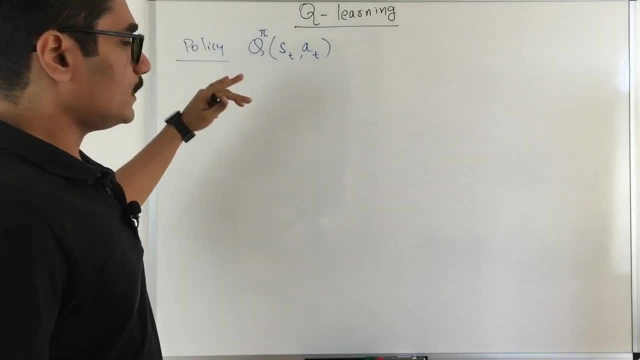 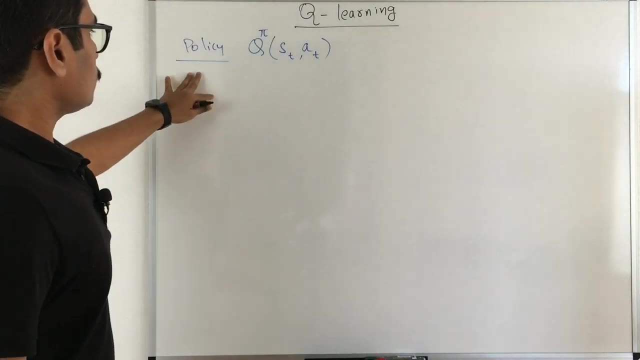 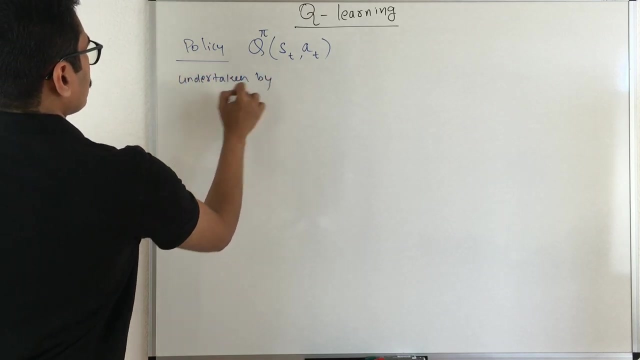 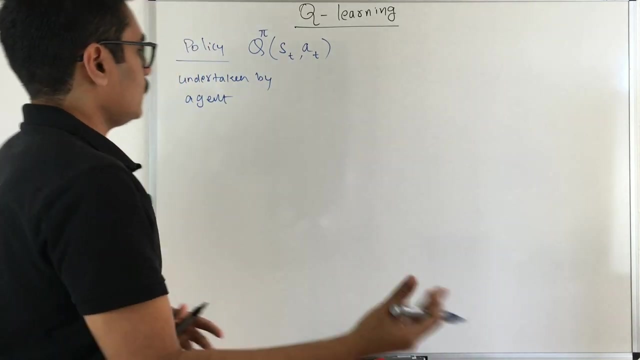 policy. So similar is the case with Q-learning also. you have certain limits, certain regulations, certain services which are to be provided, which are not to be provided. So policy is essentially undertaken by agent. So agent takes the policy and he sees in a given state. 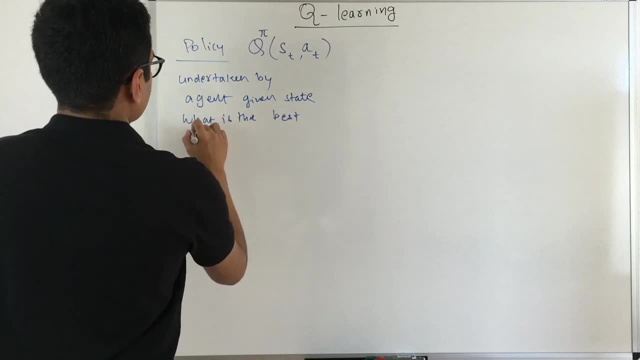 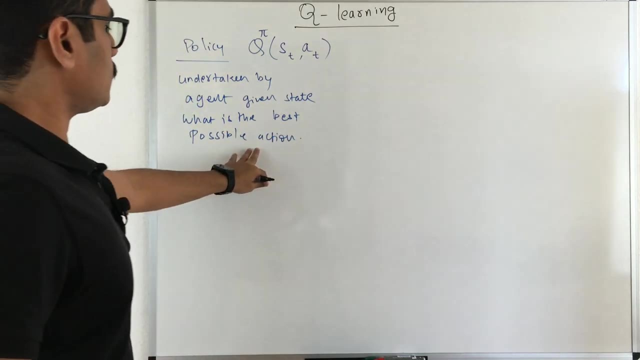 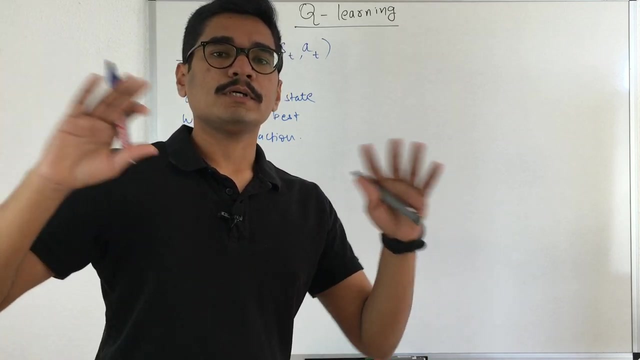 What is the best possible action? So that is simple. Let me give you an example for this. say you are on a main road that is on a lane, So just the streets are just empty. You are just the only one who is driving on that. 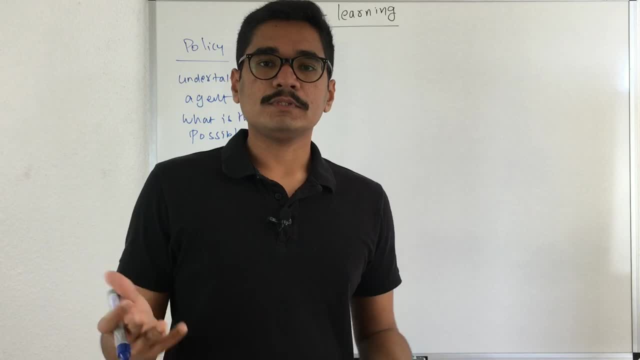 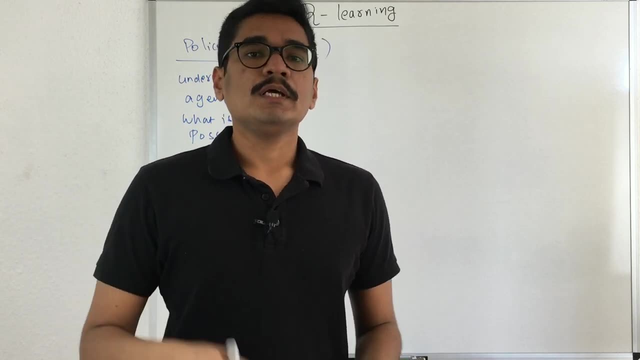 So what we will do is you will put on the top gear, fourth gear, and then you will just accelerate, and then you will just go. so there, at that point of time, no one will instruct you like you have to go on this speed or you have to apply this clutch and this stuff. 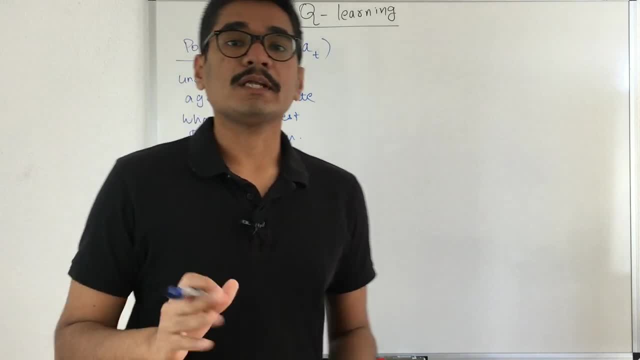 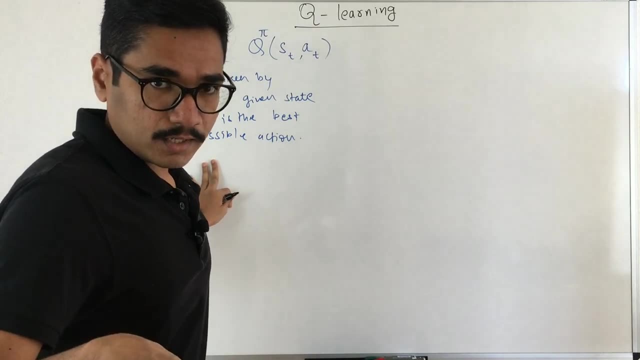 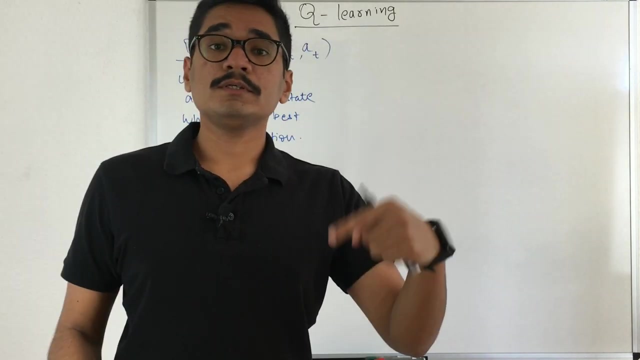 So that's it. So it's just upon you. like you'll just raise the car. So in that particular environment, your state is your car and the action that you do is you'll just accelerate at the top speed. So that is the policy you will take at that particular instant of time. but that is not. 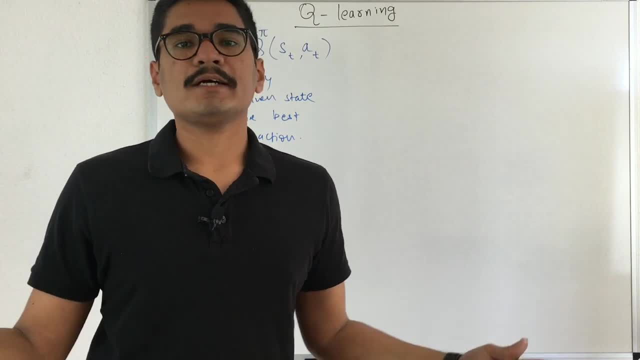 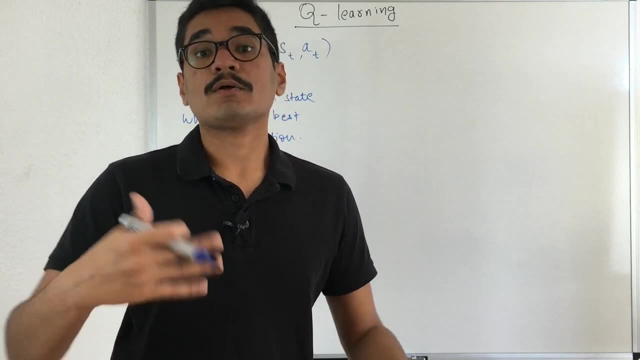 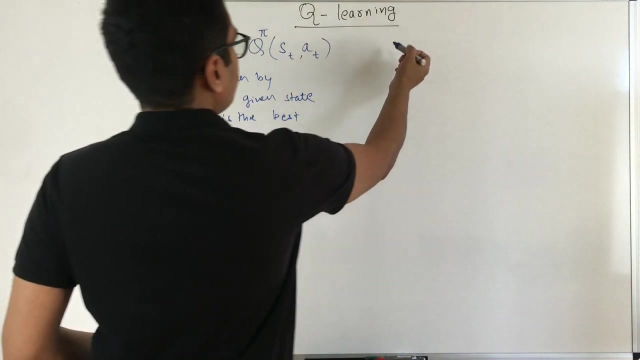 always the case. everywhere It's not like on a crowded street. you do that thing, So that is very dangerous. It's very dangerous to the pedestrians and the people who are there and also to the other vehicles. So this is one essential term inside Q learning. that is policy next term that will be discussing. 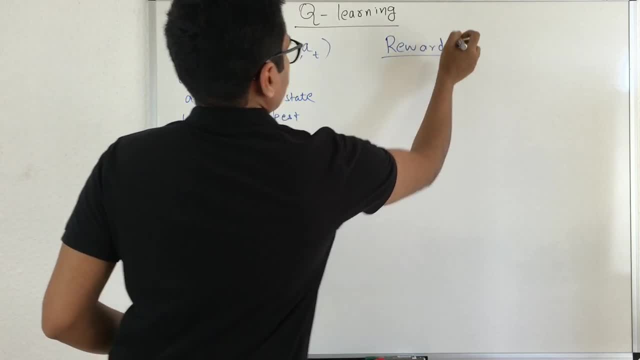 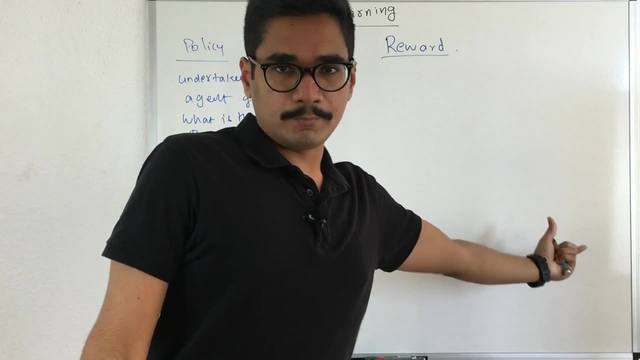 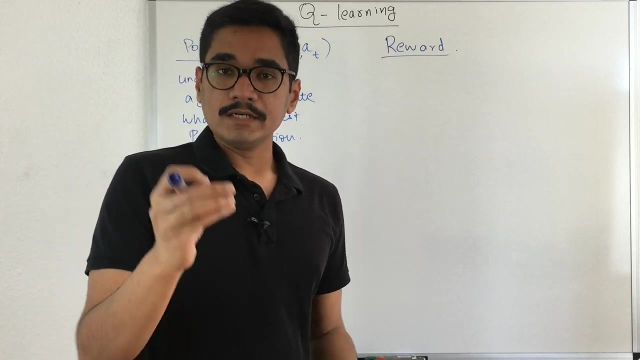 is about the reward. So reward. we have seen many times, like in the previous slide also, we have seen an apple. that was a fruit, which is considered as a reward for that particular agent. So whenever the agent is the rightful action, They will be. 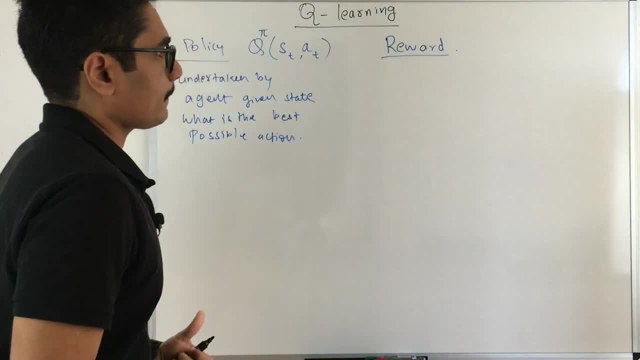 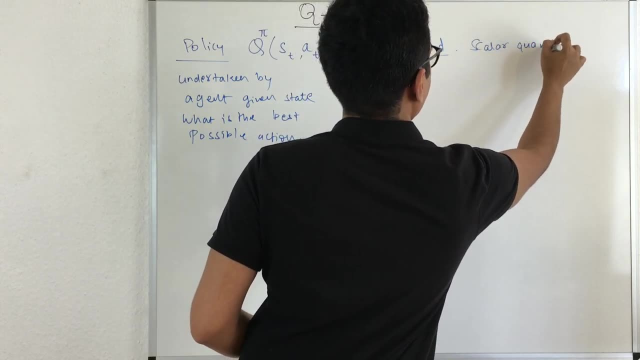 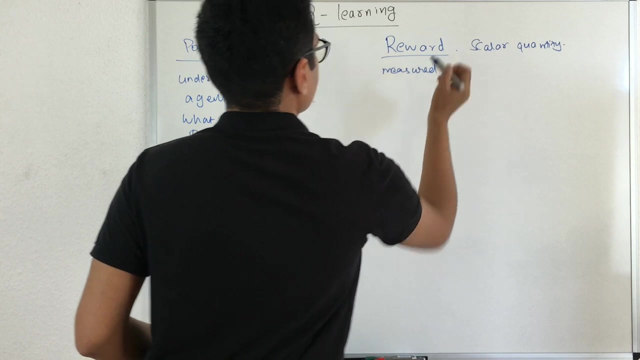 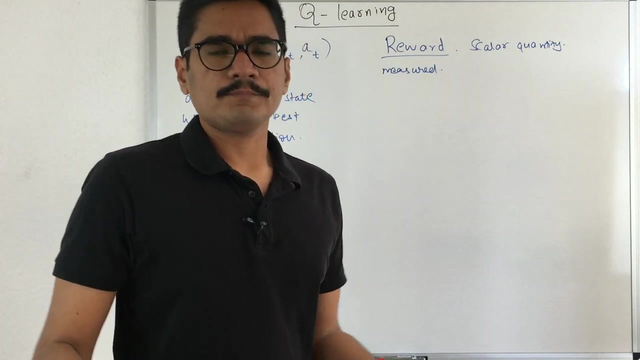 They will be awarded with a reward, that is, a gift or a present. So in Q, learning reward is considered as a scalar quantity. scalar means it can be measured, So measured in terms of some units. So usually in real life we want to buy some products or whenever the cost optimization 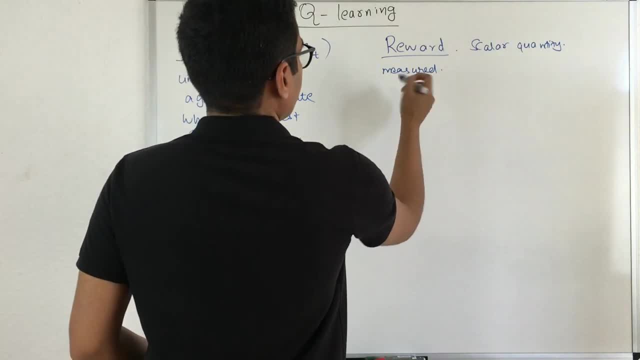 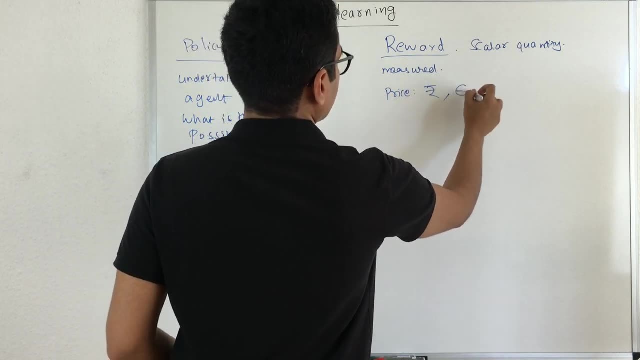 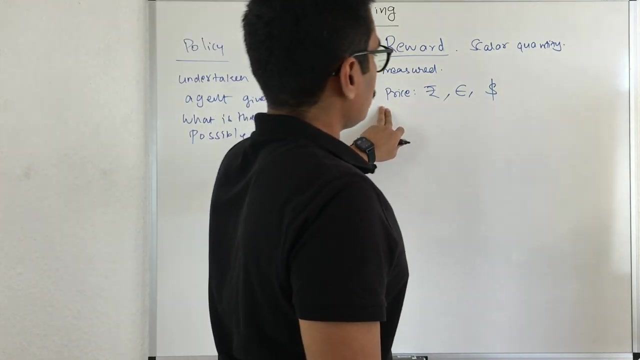 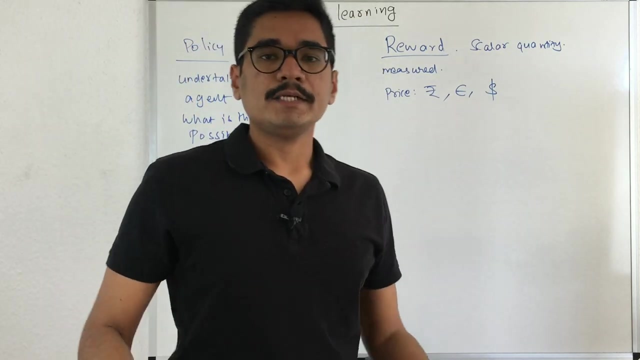 cost estimation comes into picture. We mainly use the reward of price, So it can be in any symbols like rupees or euros or dollars or any other cents which are there in the real world. Now, sometimes we can play with this reward. So if you are into a competition and if you are participating into some games or some, 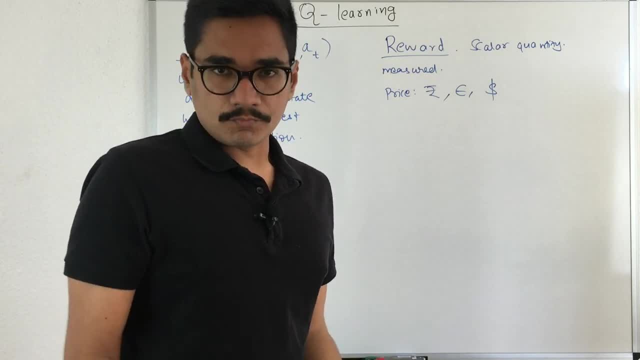 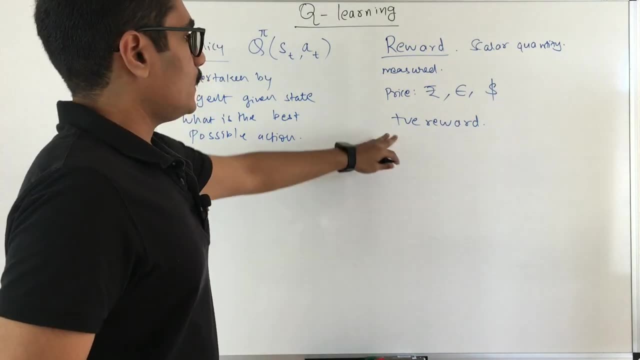 hackathons or somewhere, you'll basically get a reward. So if you are participating in a competition and if you are participating in some games or some hackathons or somewhere, you'll basically get a reward. So that can be considered as a positive reward. 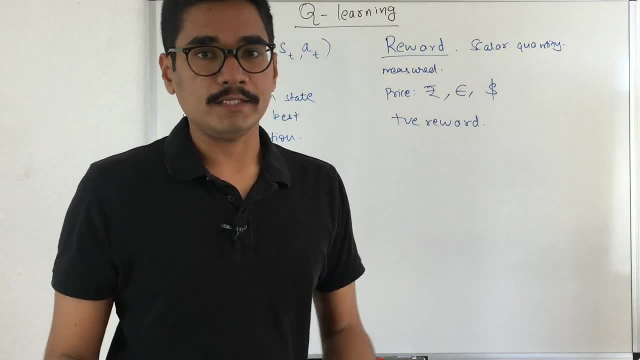 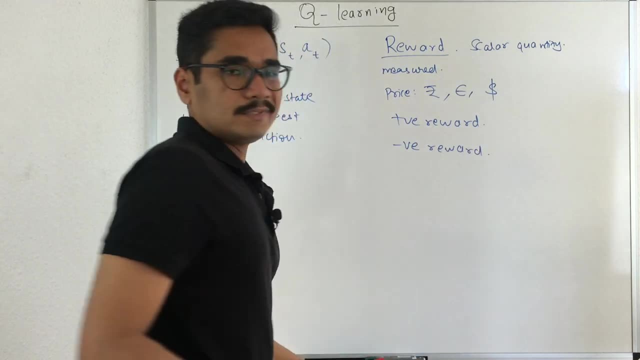 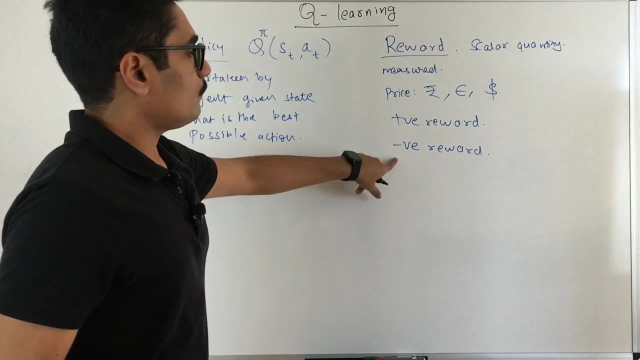 And then sometimes you also face this reward as a penalty. So that is not the reward. instead it is considered as a negative reward. So you don't use the word penalty, instead you use the word positive and negative reward here. Now, where does negative reward comes into picture when you park your vehicle at a wrong? 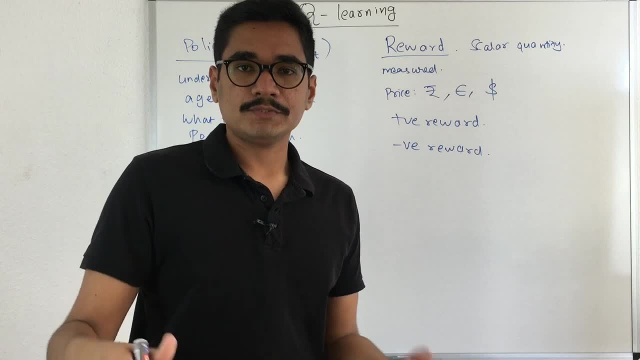 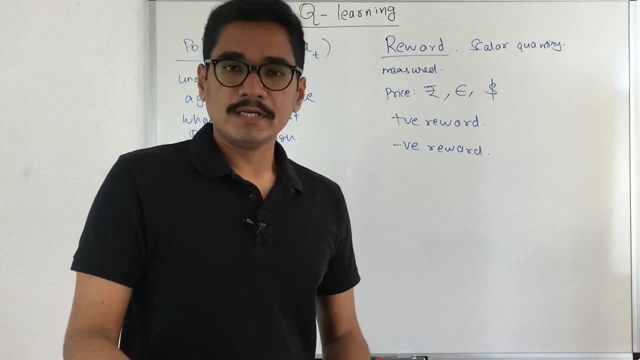 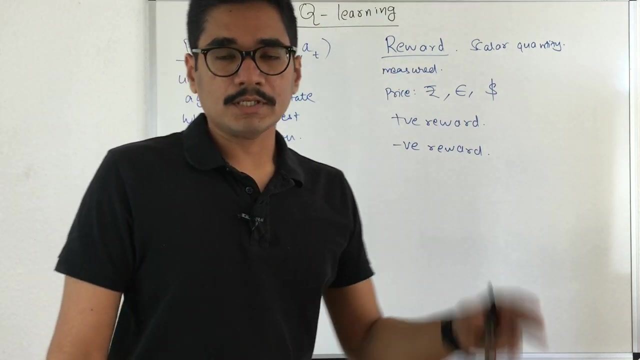 place or, if it's not, at the place to park and the police officer comes there and they just charge you. that is just a penalty they are imposing on you, So that essentially becomes a negative reward. So the same logic revolves in machine learning, agent also. so agent will face positive reward. 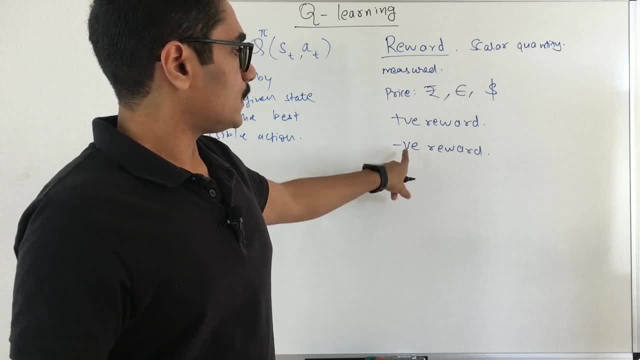 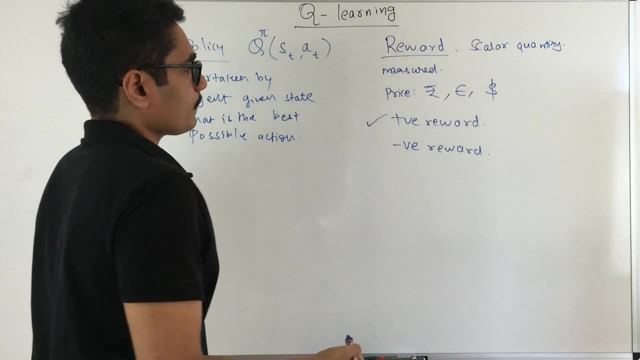 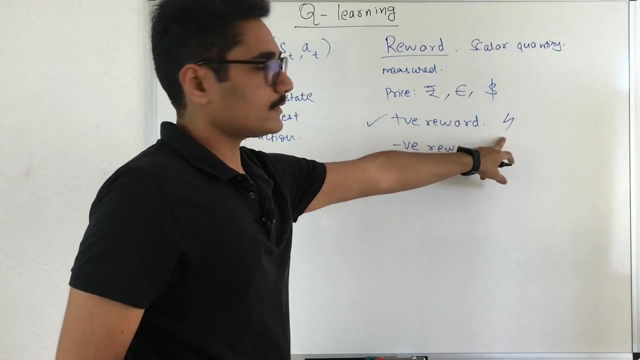 and negative reward for each of the action which it incorrectly implements. So our goal is to maximize the positive reward that we want. So reward can be considered as some energy points, So it is given as a power symbol, something like this, or it can be considered as price. 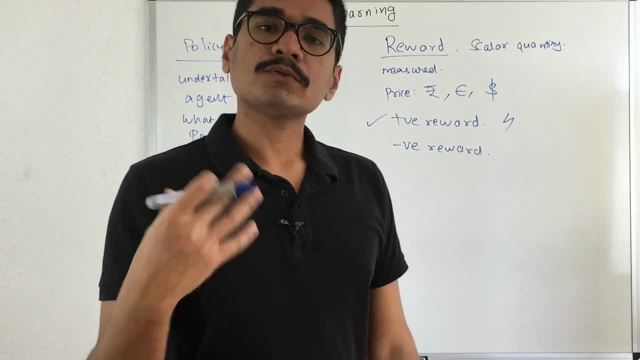 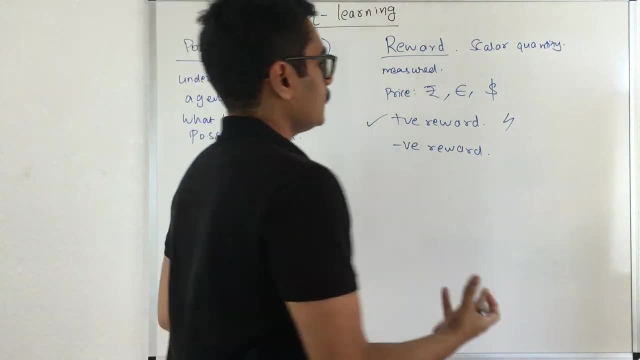 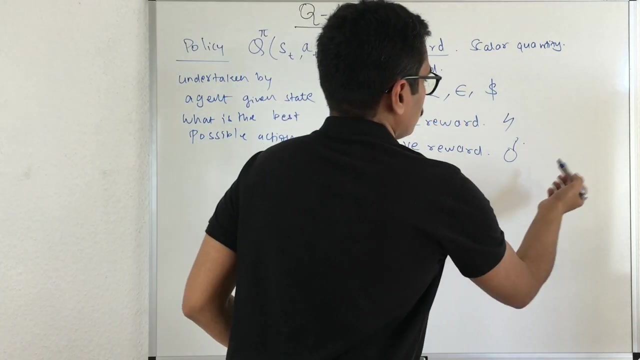 or in that example we have seen a fruit example. So all those things are considered as reward. that is positive reward, and in negative reward you have something like you have a mine, that is bomb Which Which is there. so or you may have like reducing the lives. 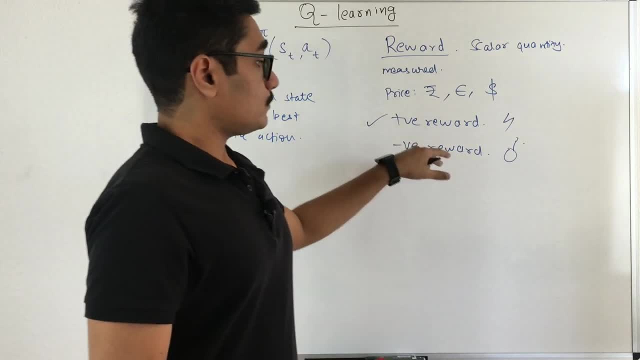 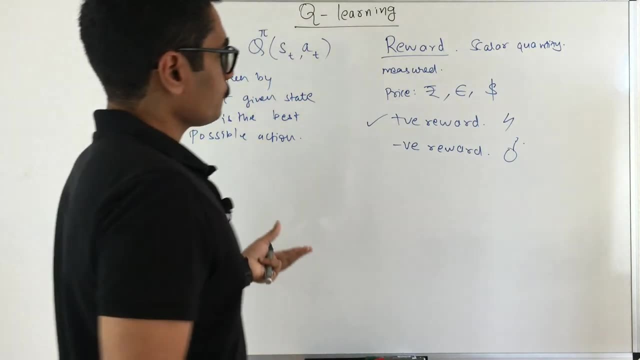 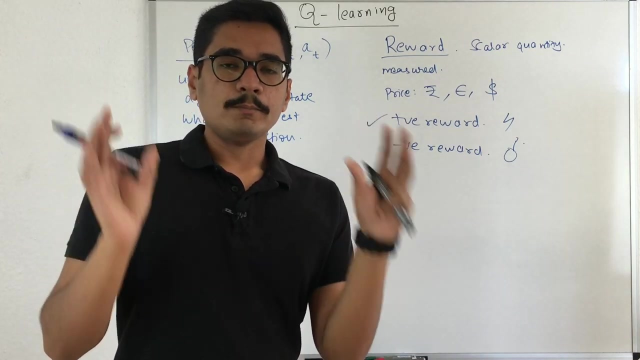 So your health may be decreasing due to some activity, So those things are considered as negative reward. So these are the two important things, apart from the state and the action which you see in Q learning algorithm. Now let us see the two main backbones from where the Q learning algorithm comes into. 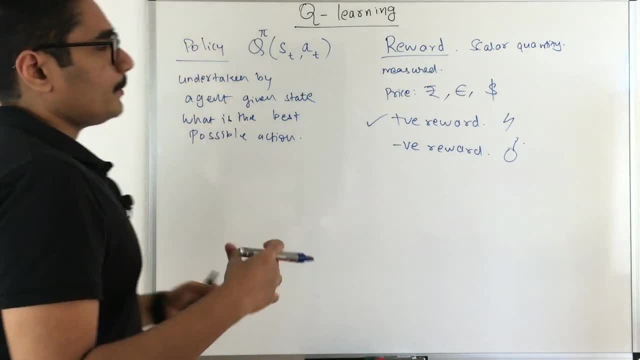 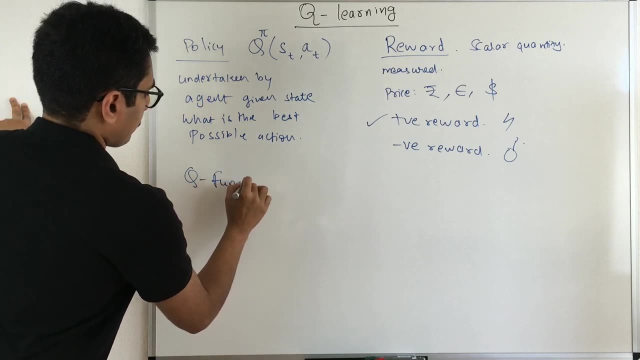 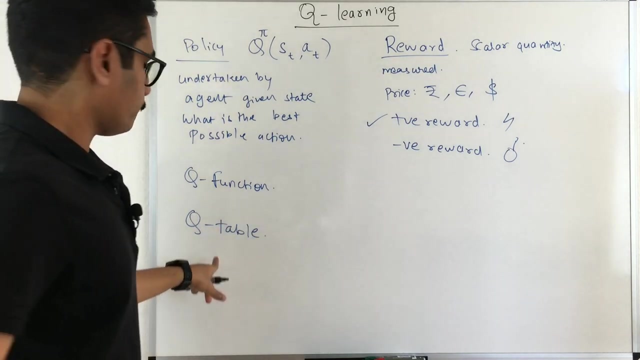 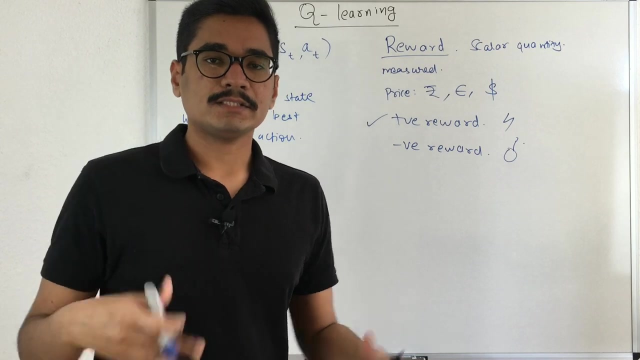 picture. So in Q learning There are two main entities, as in we can say as the Q function, and then you have something called as Q table. So you basically construct a Q table, given a set of actions and given the directions that you want to perform in that particular environment, and then you apply a Q function. 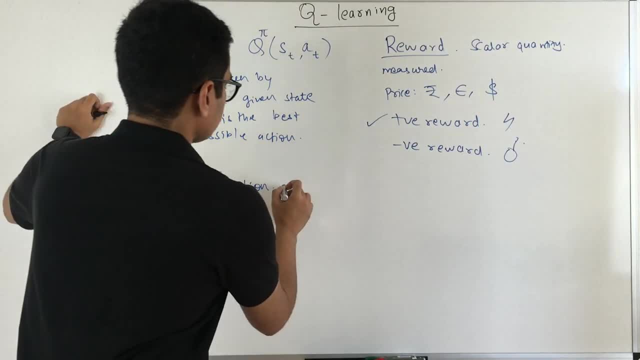 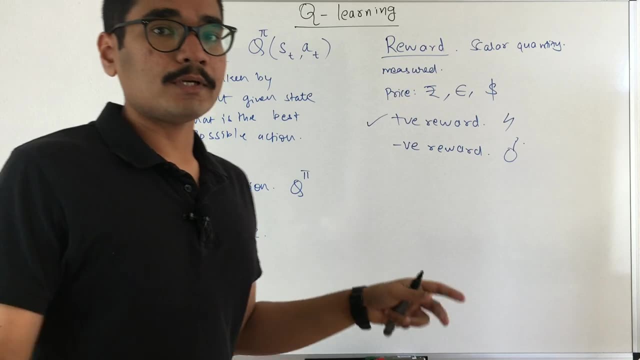 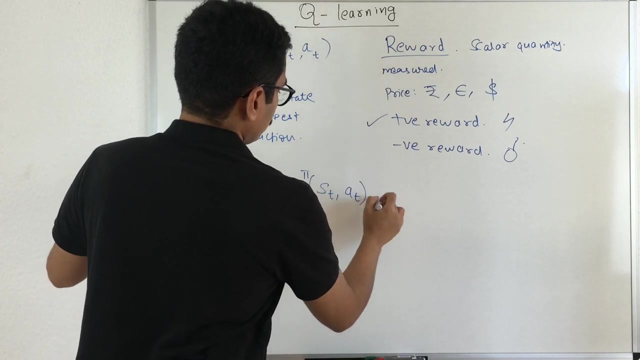 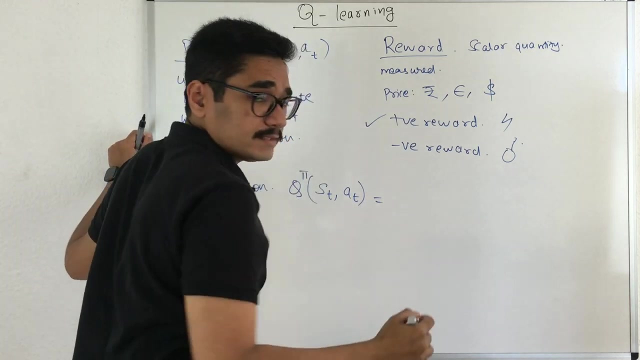 on top of this. So Q function is given As, so that takes the optimal policy into consideration, that is the best action in that particular state. So you have the state at that particular point of time and action at that particular point of time. So the Q function is written as the policy and it is the expected value of the rewards. 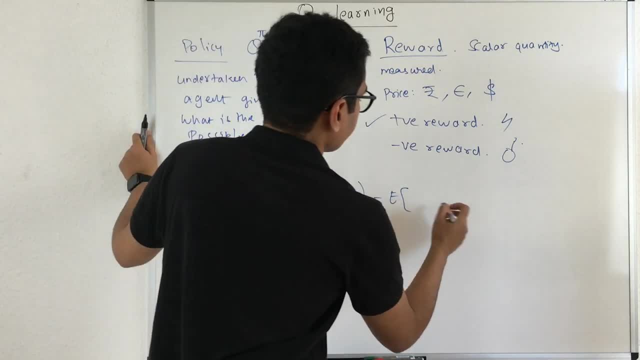 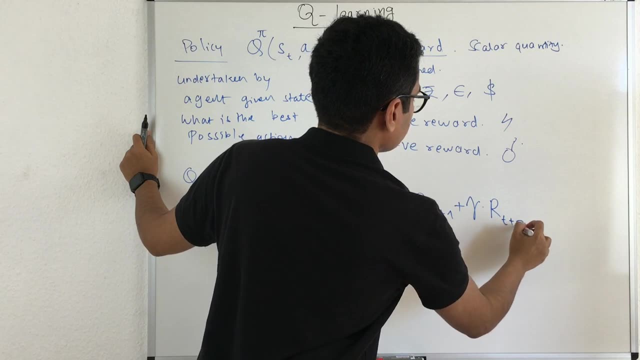 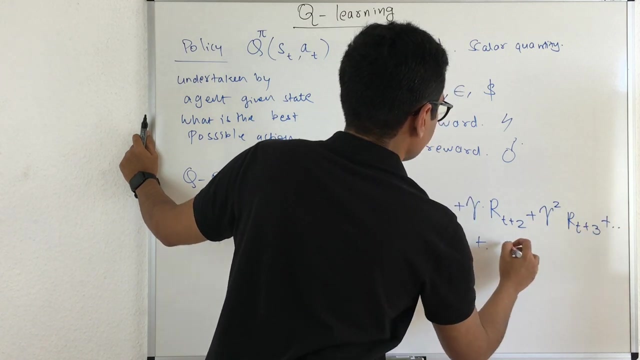 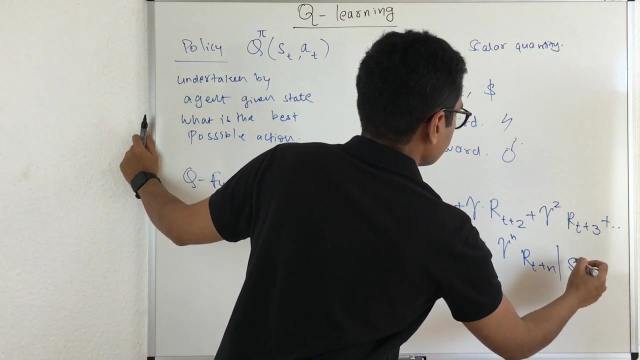 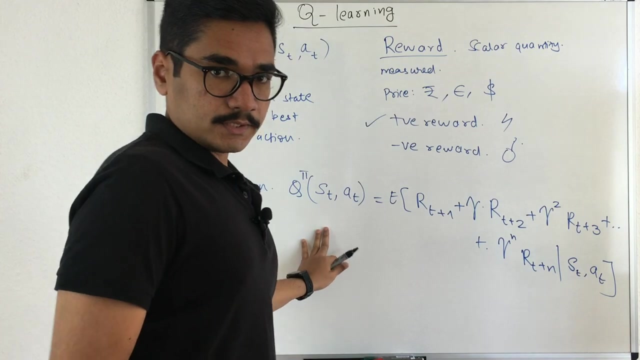 and the discounts. So it is written in this way. So you have RT plus one Plus Gamma, RT plus two plus Gamma Square, RT plus three, up till you have Gamma n, RT plus n, such that you have ST and 80. So this is the Q function that you mainly use in Q learning and this particular equation. 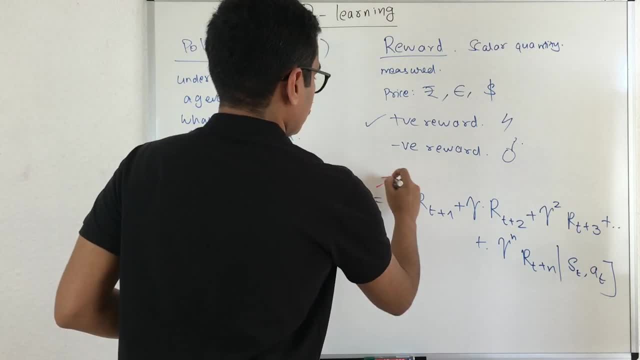 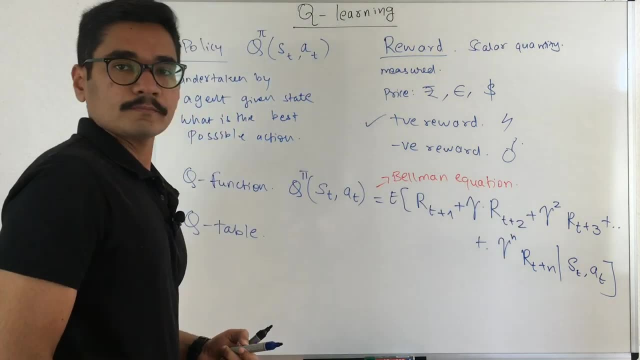 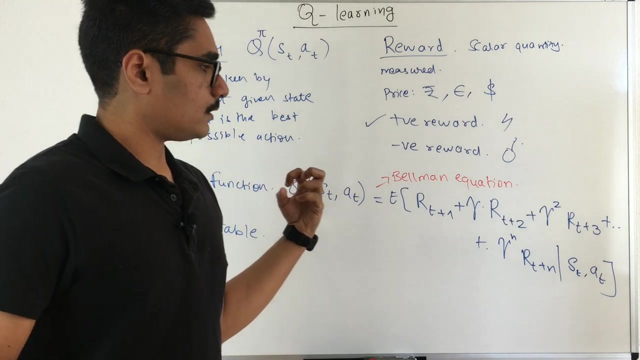 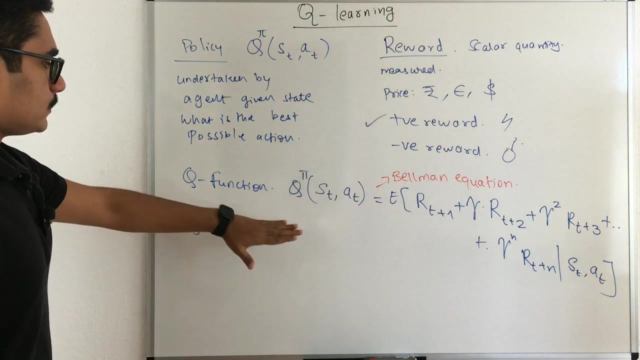 which you see here. This is called as the Bellman equation, So this you essentially use in Q learning. So this is the actual mathematics or the power from where the Q learning algorithm learns. that is the Bellman equation. So that is one component of Q learning. 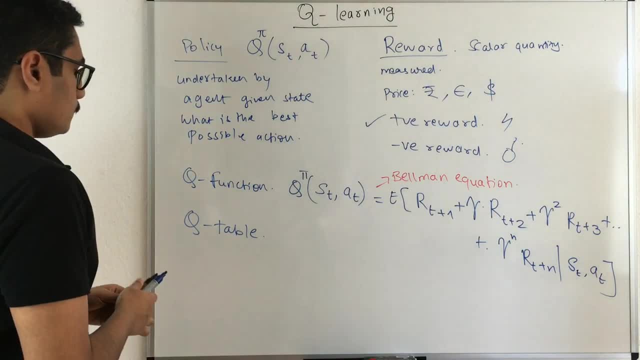 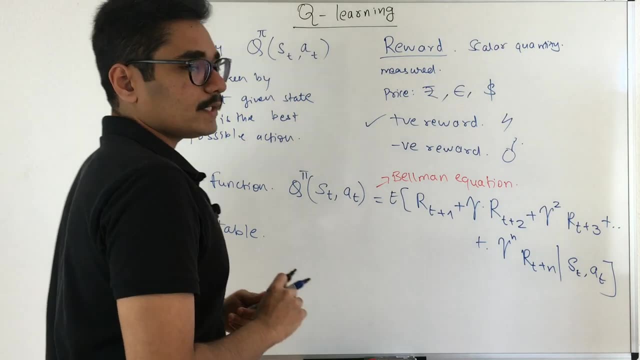 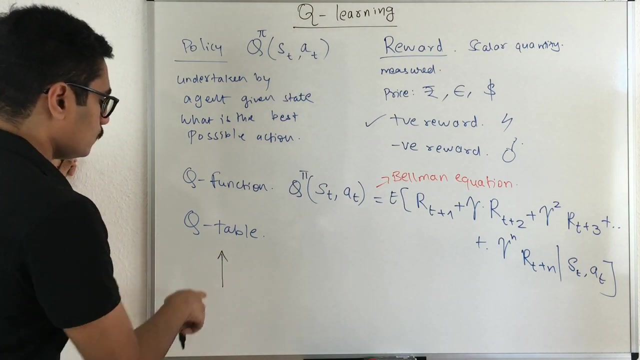 Then you have something called as Q table. So in the maze problem which we saw in the beginning of the video, there were only four possible actions that that turtle could take. So it was: either it can move in the top direction, or in the bottom direction, or on the left. 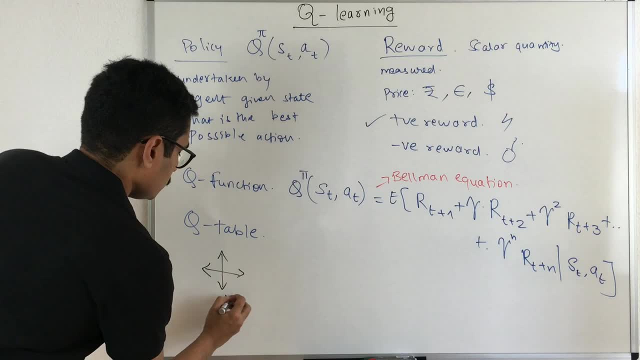 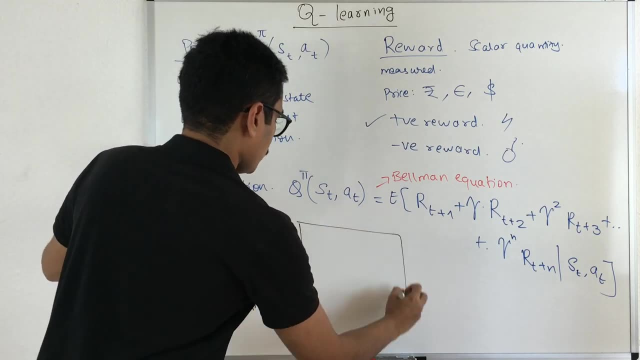 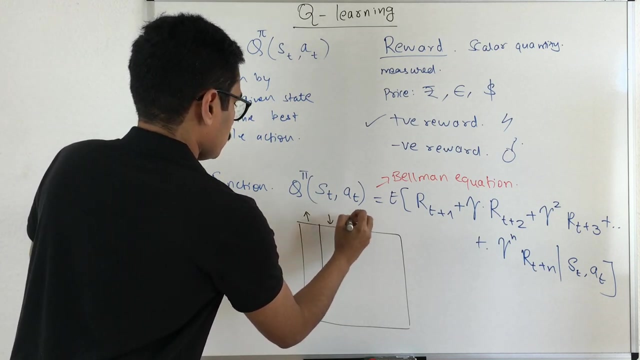 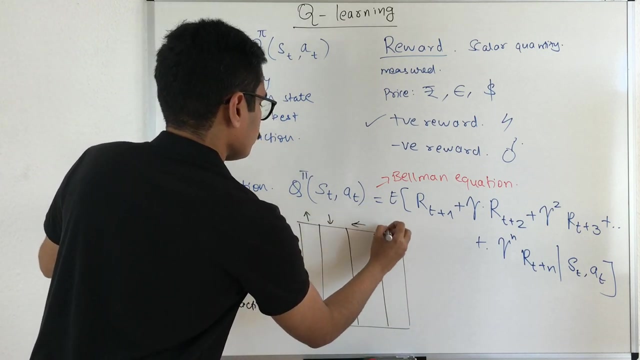 side or on the right side. So these are nothing but your actions. Okay, Okay. So in Q table, what you basically have is you have a table that comprises of the actions. So actions: here are all these letters up down, left and right, and what on the rows comes. 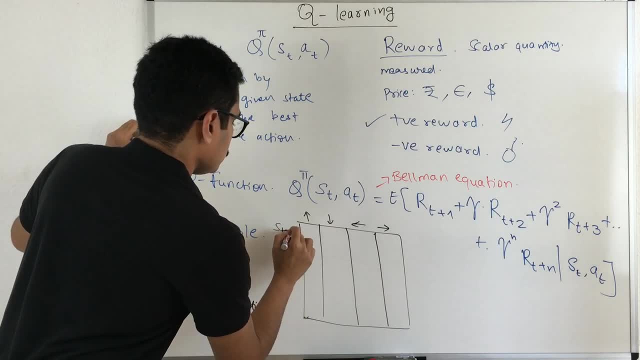 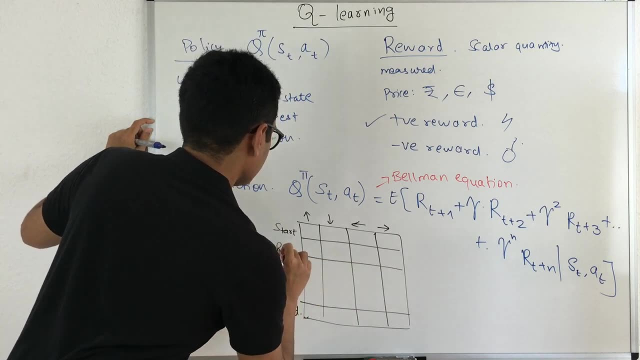 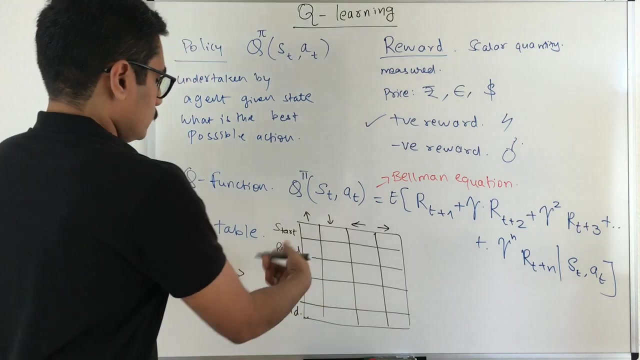 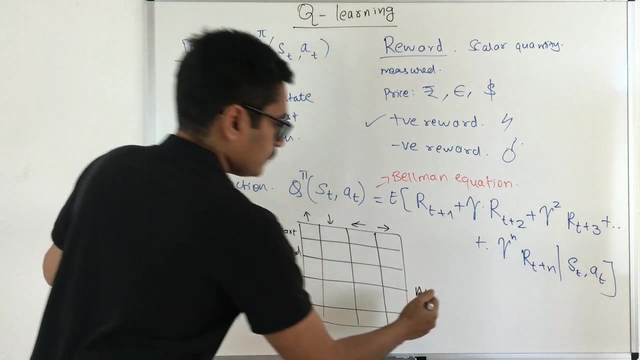 this on the state. so status say this is the start state and this is the end state and you have The reward okay. and then you have some states like it is health minus minus, that is, the health decreases. So Q table is essentially a matrix, given the number of rows, that is, the states and the 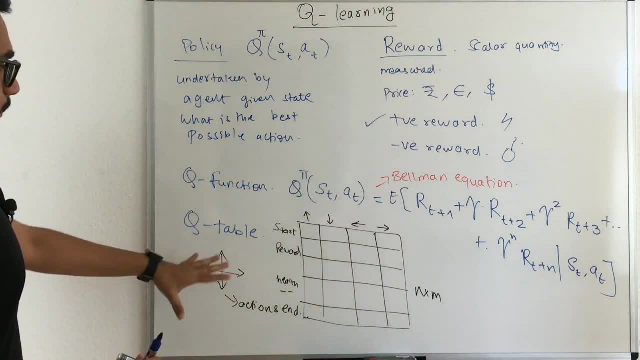 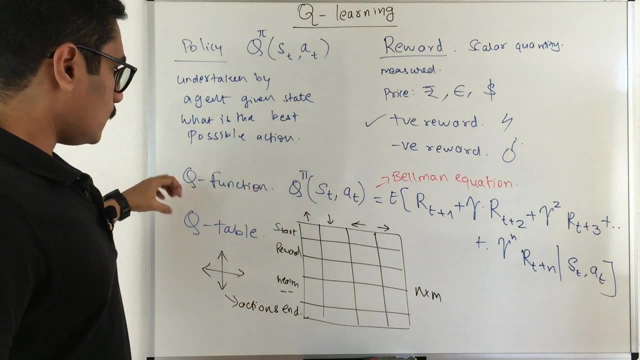 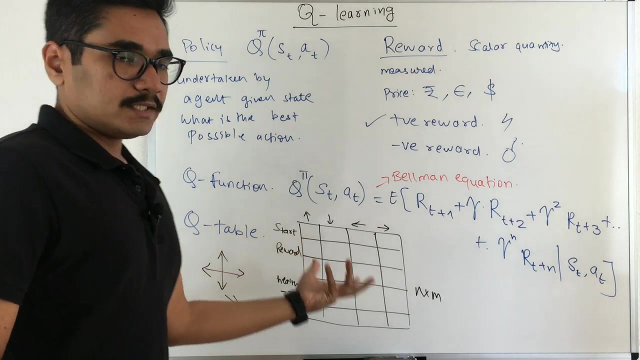 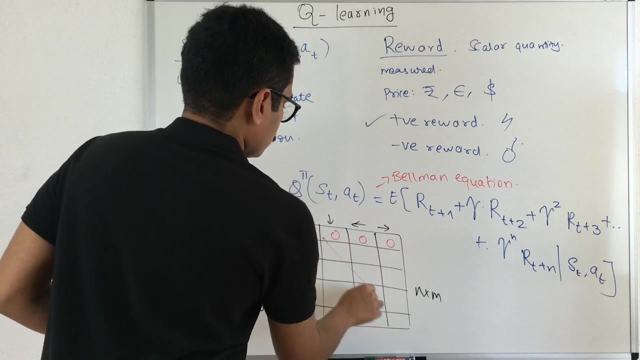 columns, which corresponds to the actions. So these two are the two components which are seen in the Q table. So you need to make out this equation first and then you have to fill this Q table. So when we initialize this Q table at the beginning you fill all the values with zeros. 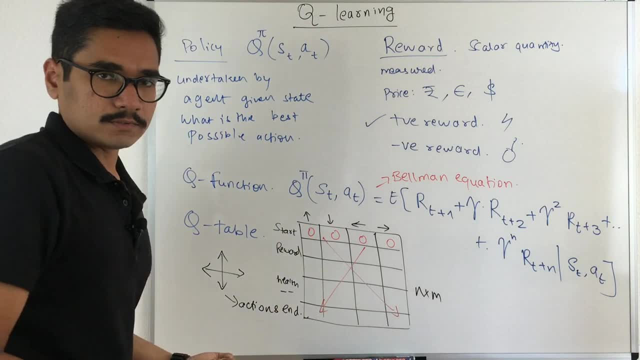 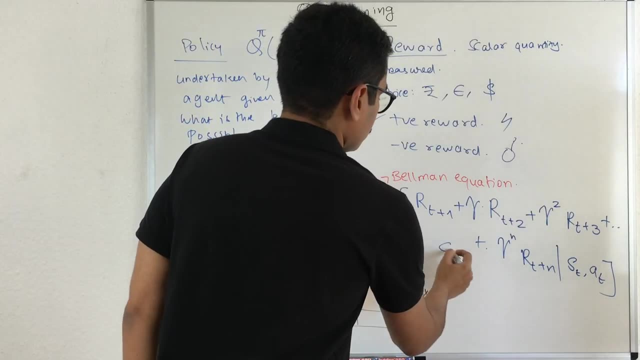 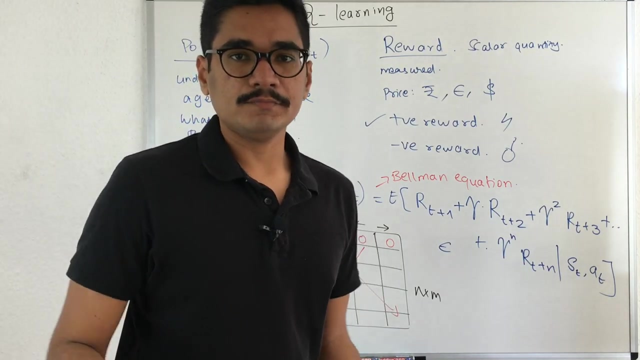 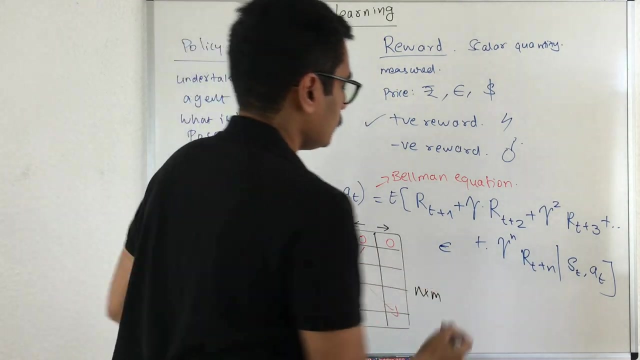 So all values are filled with zeros here, and then you have some parameter, so that parameter is called as epsilon, So which is a hyper parameter. So hyper parameter is something that we introduce explicitly, which is not already present. So, since you introduce a hyper parameter that is epsilon, this follows a strategy called 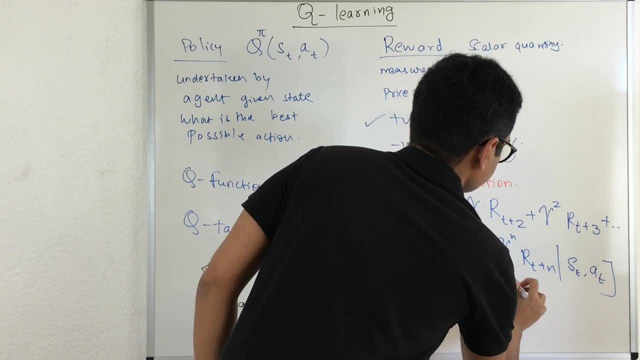 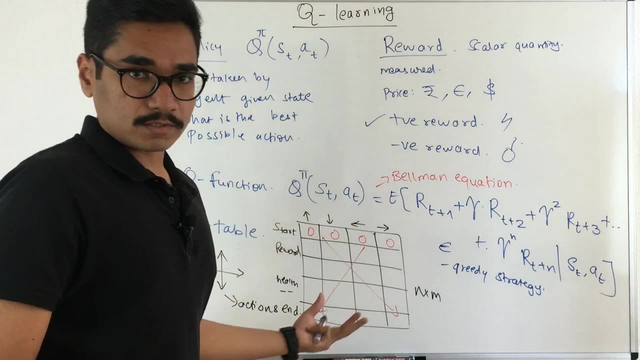 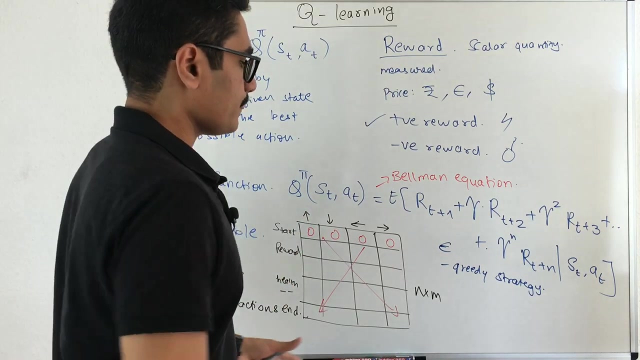 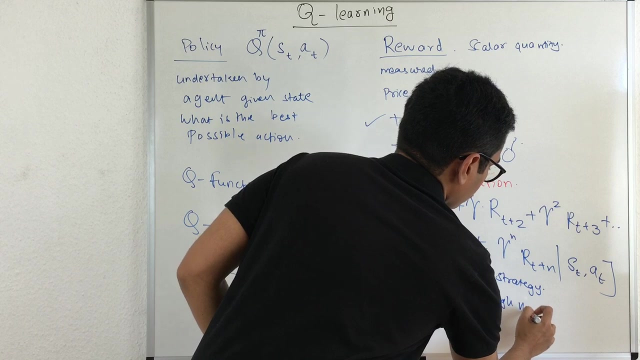 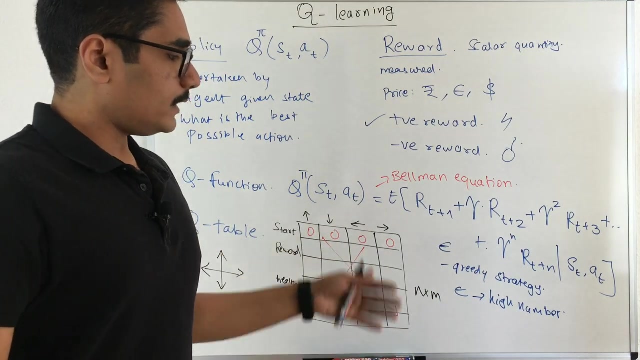 as the greedy strategy. So initially, when you just initialize or start the Q learning algorithm with all the Q functions- Okay- And the Q table with all the values initialized as zero, you start this Epsilon values with a very higher number. So first you initialize this Epsilon value to a higher number, then when the agent learns, 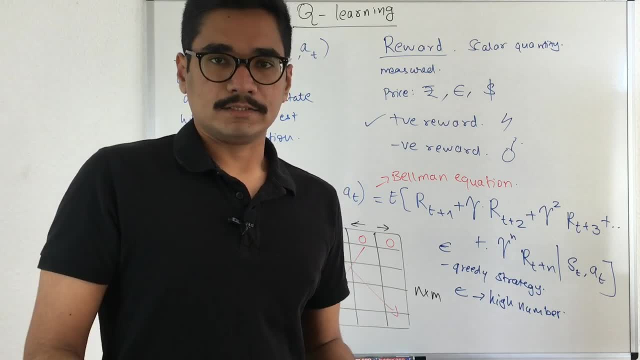 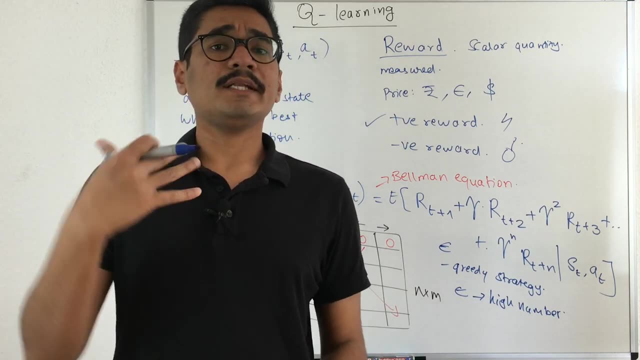 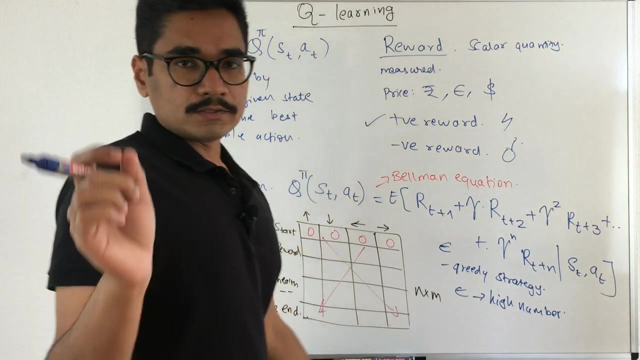 here and then now. then you try to decrease it accordingly. So that's how you do the reinforcement learning. It's not a one-time activity. It's an iterative, recursive approach that you follow every now and then at every time period. So this brings us to a discussion. that is a small discussion, which is seen here. 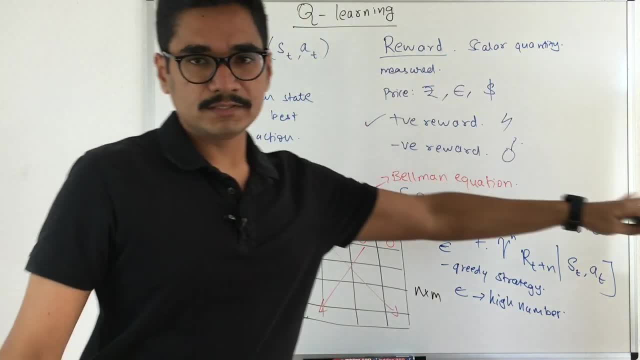 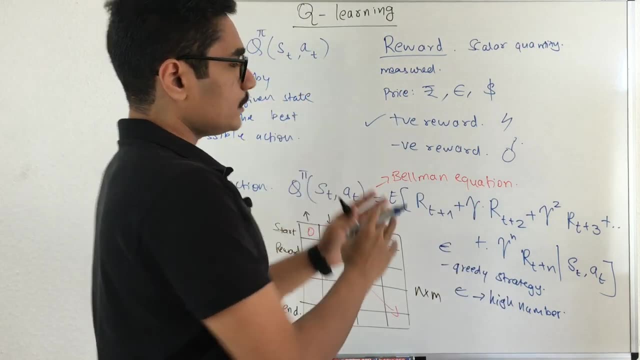 So whenever you do the Q learning or whenever you have a maze that you want to solve, So basically, first and foremost thing, what you see is the exploration, So all the possible paths that are there, that you first need to have an idea. So first thing is called as: 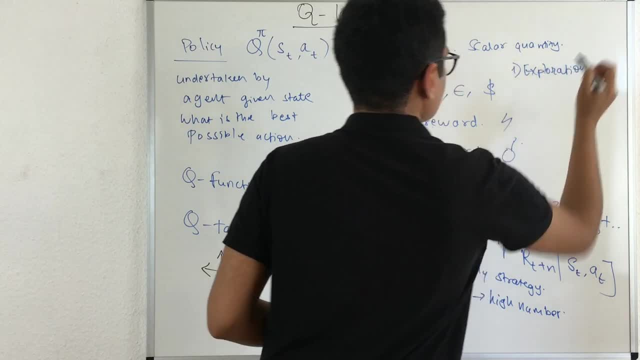 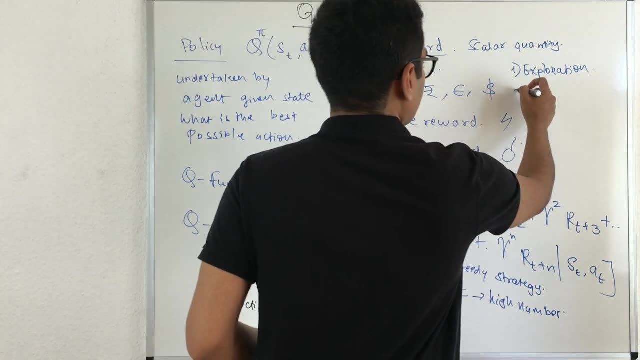 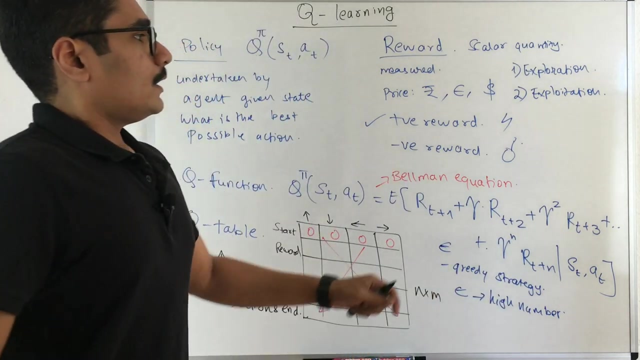 Epsilon Exploration. So first you will explore what are the possible available paths that are there in your system and then, once you have done that, you will do the exploitation. Exploitation means the best possible path which will take you the minimal amount of. 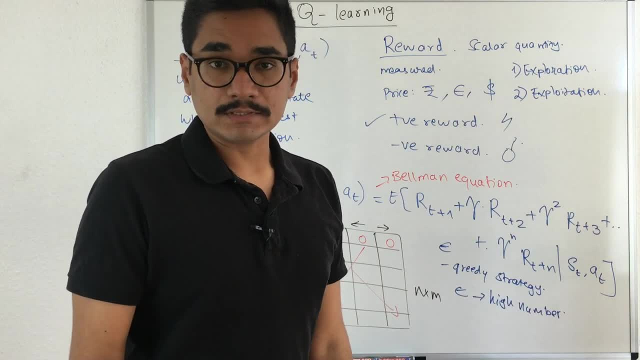 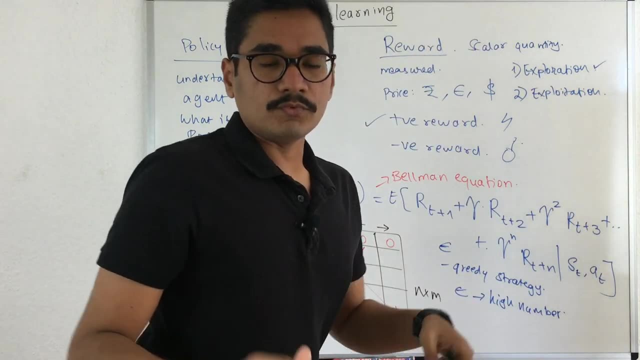 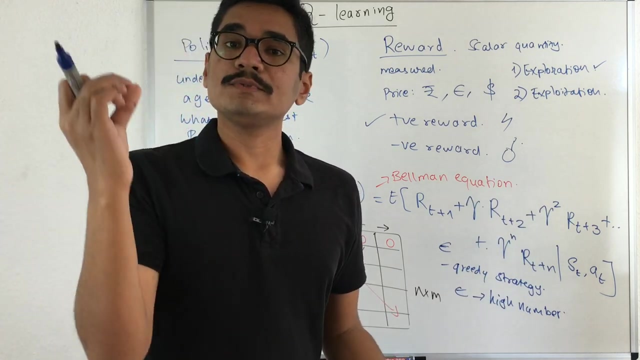 time to reach the reward, or take the reward that you want to take into consideration. So these two things go hand-in-hand. Okay, But essentially, first thing is exploration: first to explore the entire map or the entire maze that is there in your present scenario, and then you'll choose the best, optimal path. 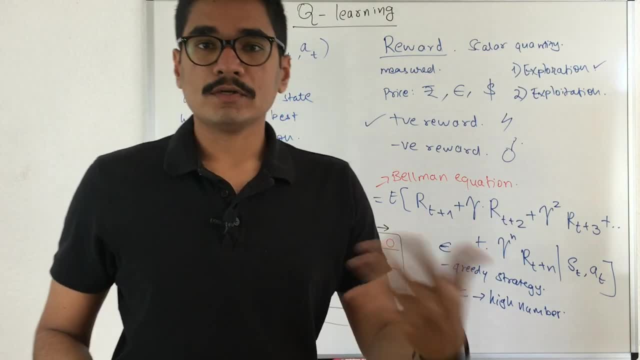 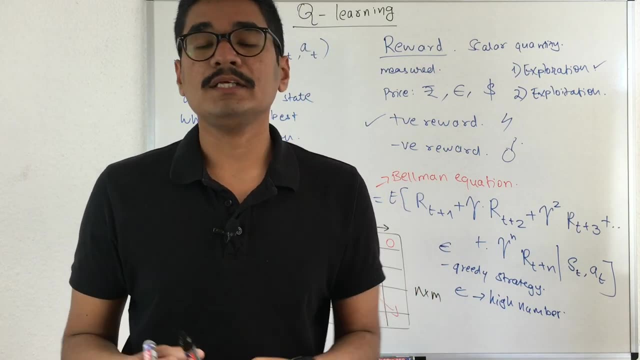 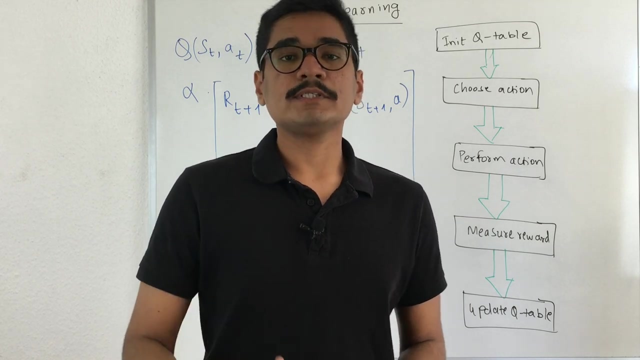 to reach your destination. Now we'll see the main algorithm, how the Q table is updated or the Q value functions learns, and from where the rewards comes into picture. Okay, So now, since we have learned about what the Q function is And the Q table is, will have a list of steps that we want to perform in the Q learning. 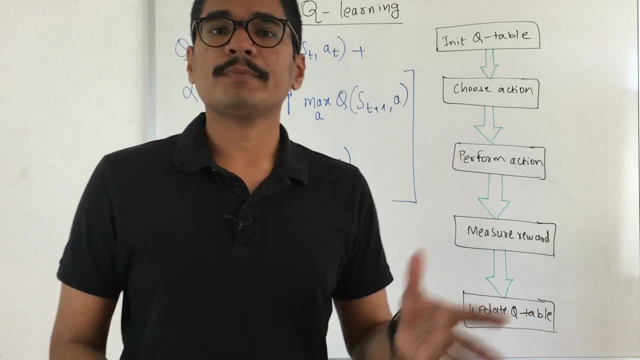 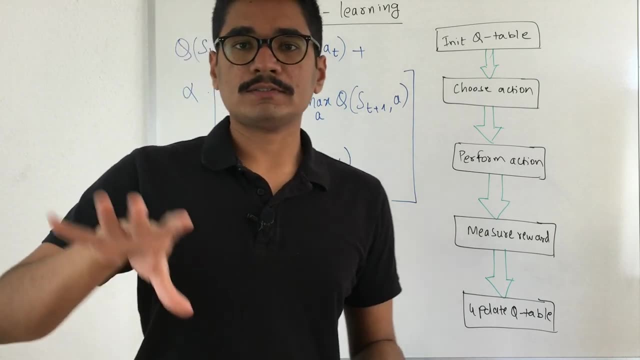 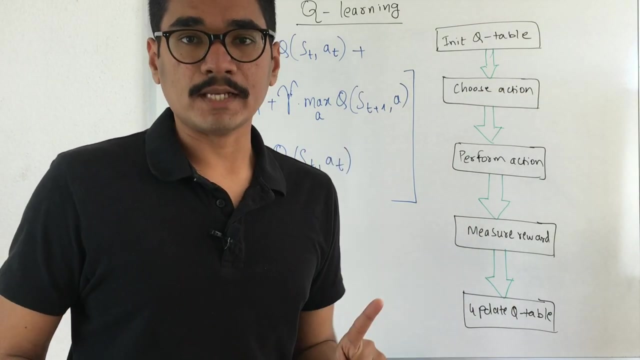 So first we initialize the Q table, So that's comprises of the states in the rows and the actions in the columns. that is a n cross m, state cross actions Matrix. that you have. then, out of all those possible actions, you will choose only one action. 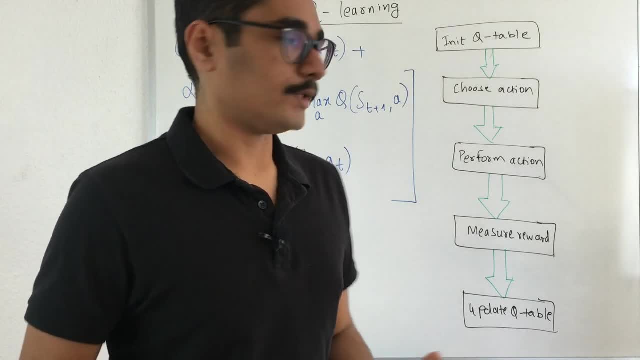 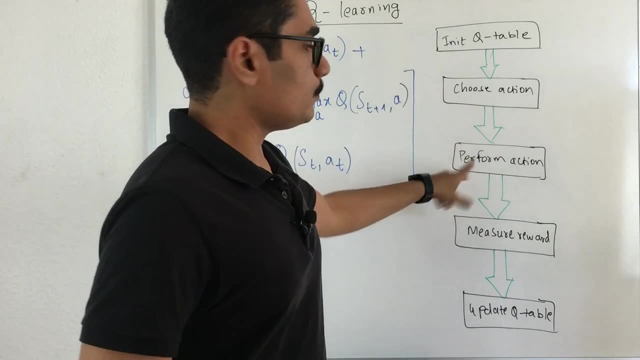 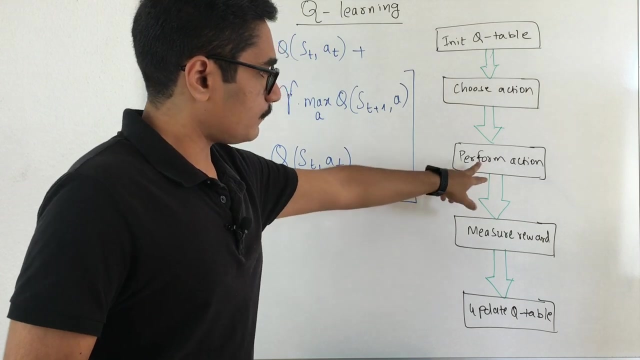 So, remember, you choose only one action at one particular point of time which is appropriate, Okay, In that particular time period, given that particular state. then you perform that taken action which is chosen from the step 2 and finally, if there is a positive thing, that 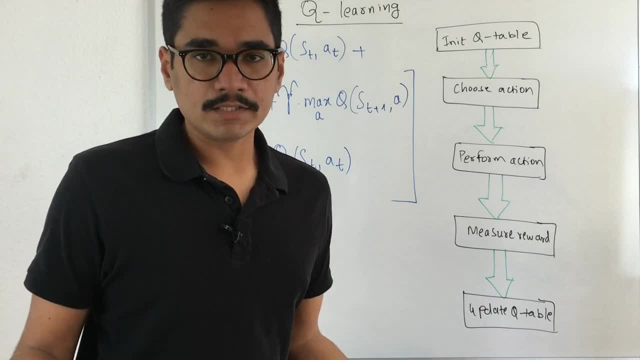 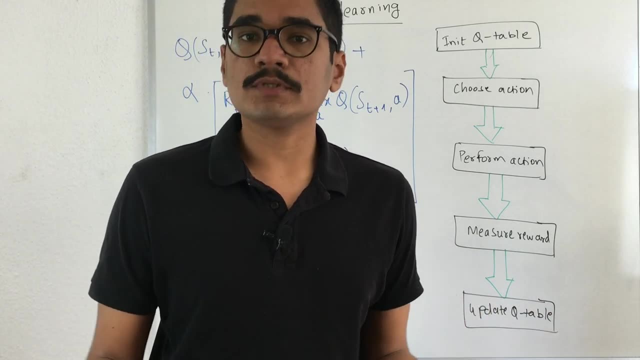 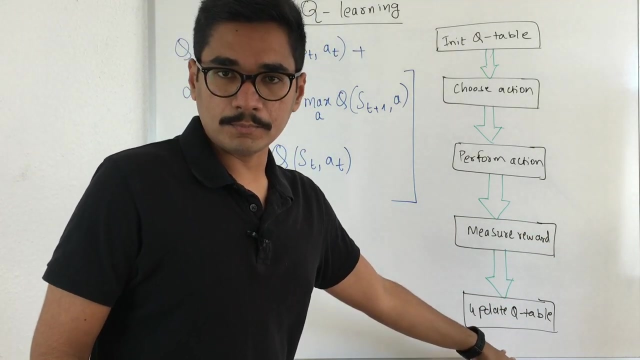 is happened, then you get a reward, else you will get a negative reward. that is a penalty. then you have to measure the reward, how good that reward is, how much future steps you want to make. so you basically measure the reward, Okay, And finally you update your Q table and then you just do the iteration of this particular 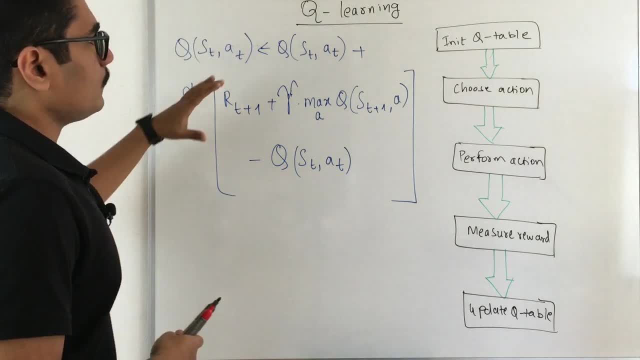 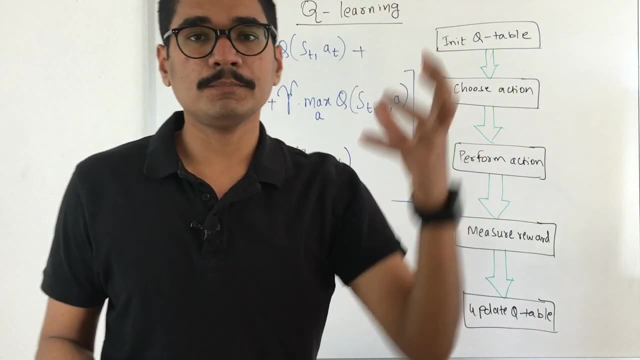 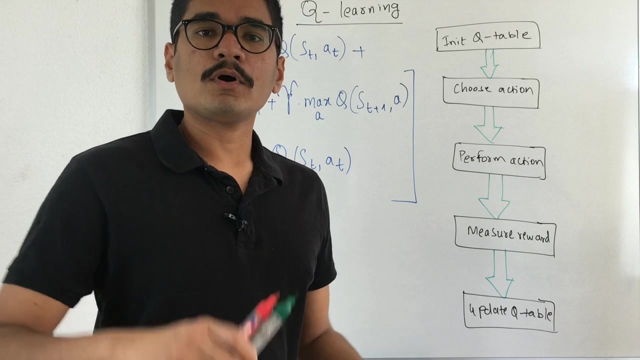 steps again and again. Now we have seen what is the meaning of Q, that is the quality. So quality is nothing but the best possible action which you take at that particular state. And then you have the learning. So any algorithm, or let it be any machine learning algorithm, we have seen the gradient. 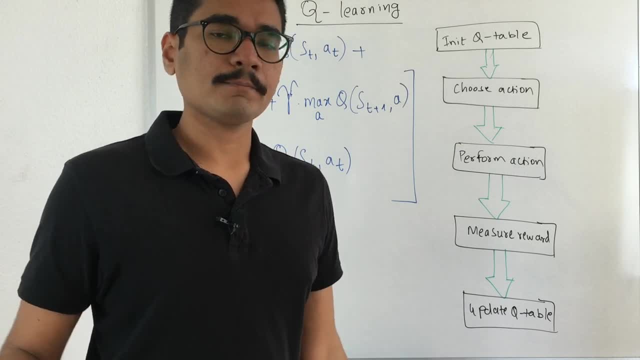 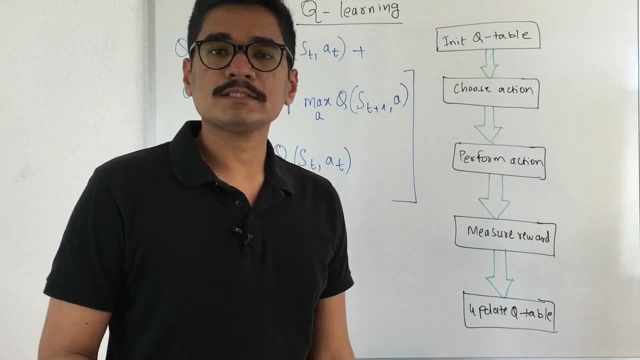 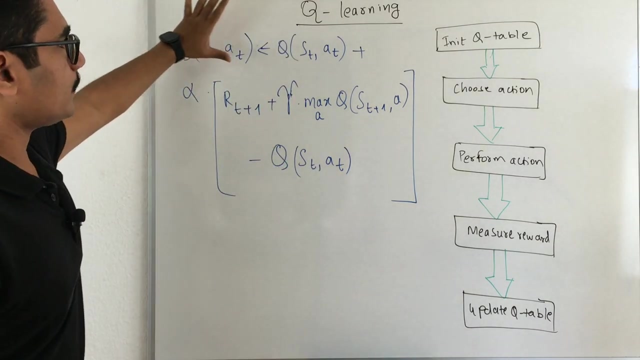 descent or linear regression, logistic regression, Okay, In anything these all algorithm basically learns. So, essentially, there is some mathematics which is there behind this, or there is a common backbone which is present in all these algorithms. So this is the equation by which the Q learning algorithm learns. just don't get frightened. 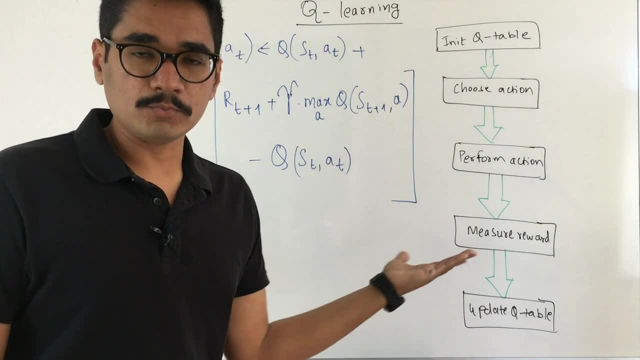 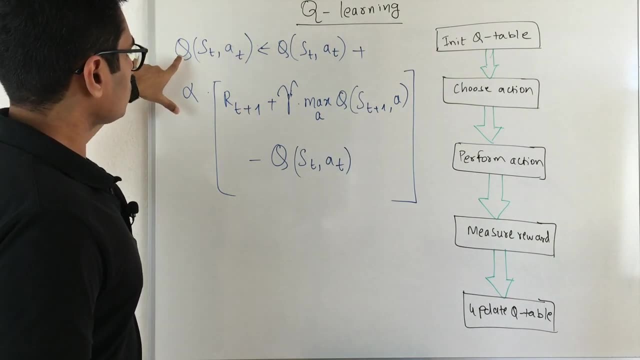 with this algorithm or the with this equation. that is very simple. So on the left hand side, what you can see is the Q value. So Q function is a parameter or takes two things: that is, the state at given point of time, and then you have the action at that particular point of time. 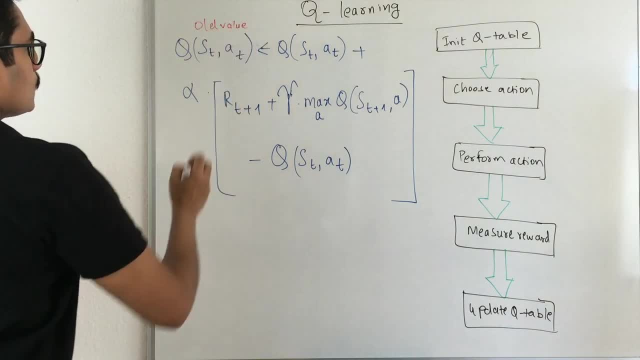 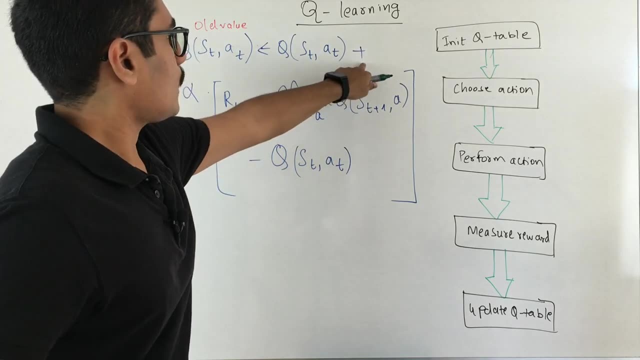 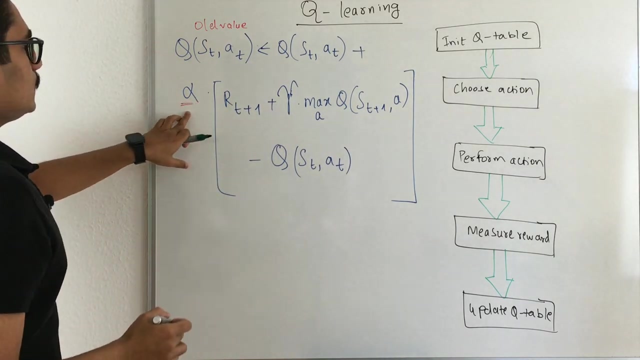 So this, essentially, is the old value. Now you have to update this old value. So, for updating the old value, you again take the old value here and you add with something here which is there in the brackets, Okay, So this thing which you see here, this is Alpha. 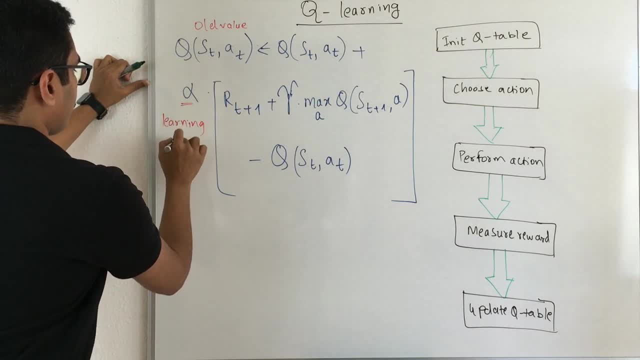 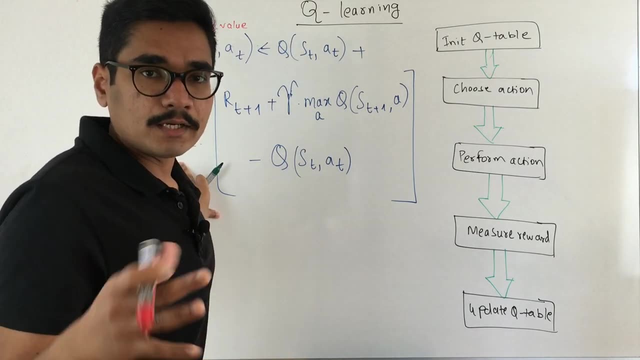 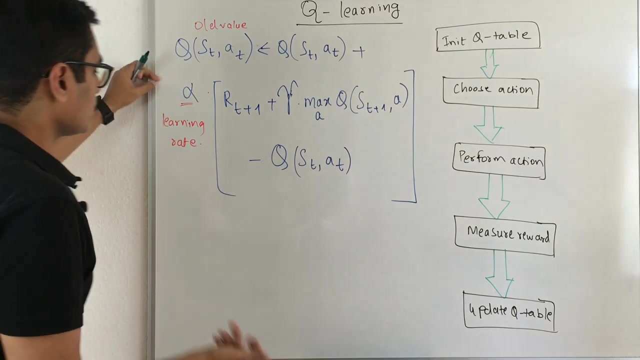 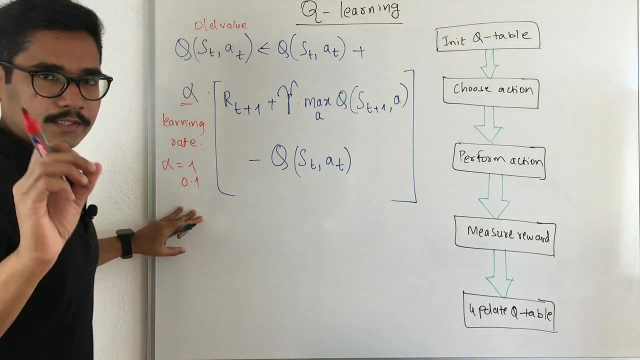 This is nothing but your learning rate. So the same thing. you have seen the gradient descent algorithm, you have Lambda, you have Alpha, So the same thing is followed here. that is Alpha learning rate. That is how much you want to learn. So usually the Alpha value is taken as 1 or 0.1 in this range, very little, small baby steps. 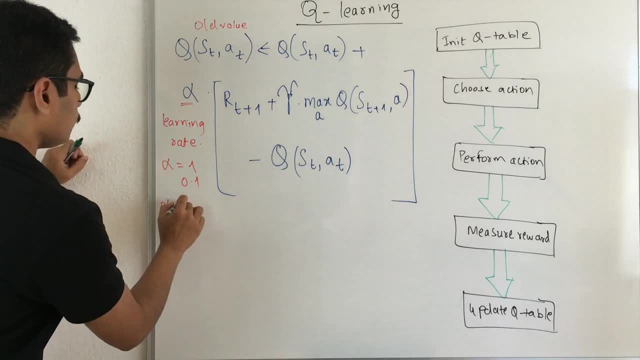 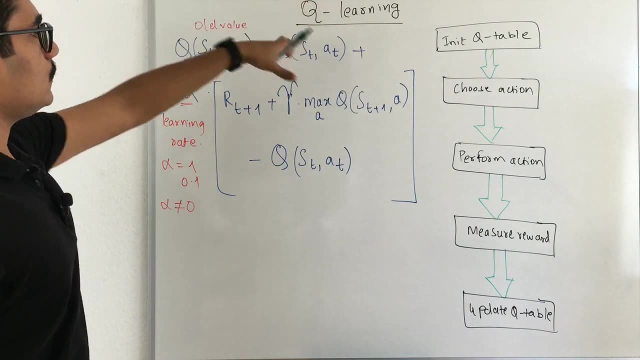 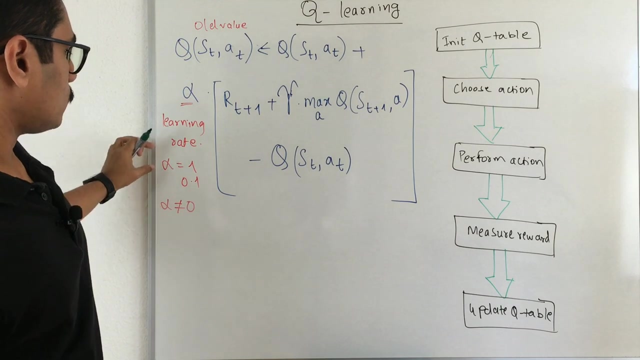 small. But you don't take Alpha as 0. if you take Alpha 0, that means the old value is equal to the new value. So basically you are not learning anything that particular stage. So you don't go with Alpha is equal to 0. instead you take Alpha is equal to 1 or Alpha is equal. 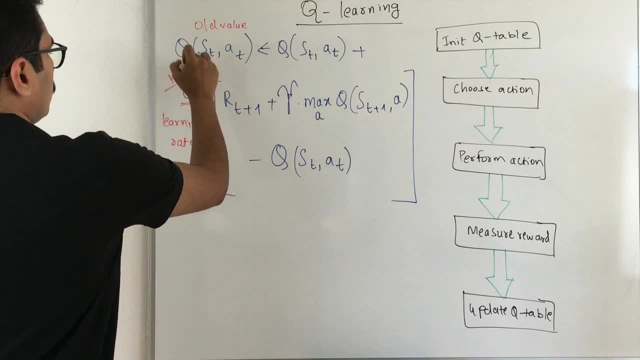 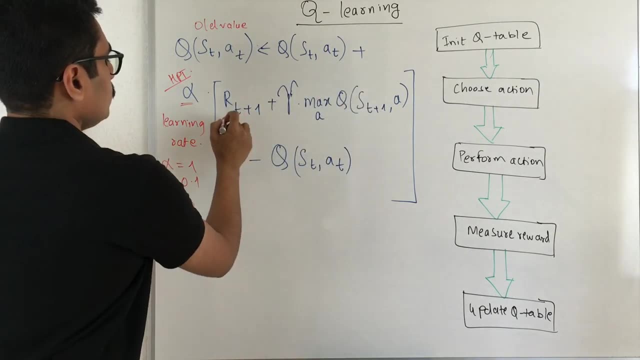 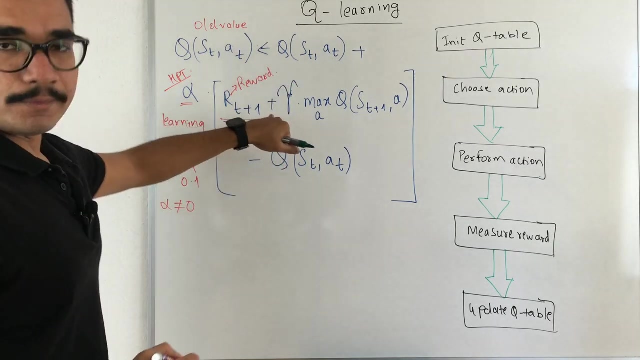 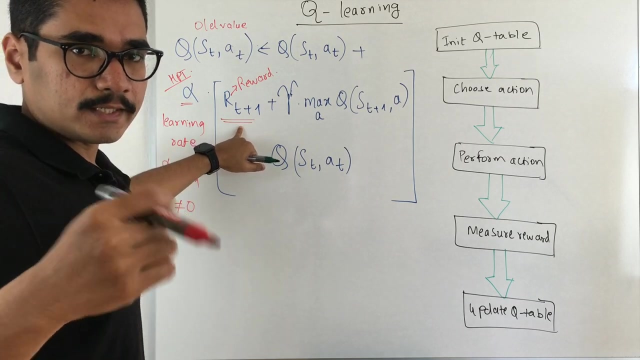 to 0 again. This is a hyper parameter that you have to tune according to your scenario. then comes the thing which is there in the brackets. So the first thing is called as the reward, So reward at time period t plus 1.. So initially from time period t you went to t plus 1, which is incremental at each point. 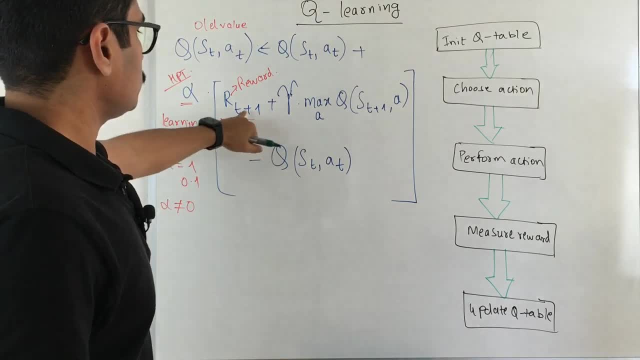 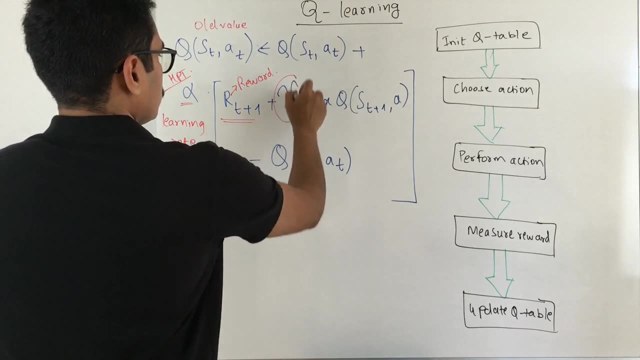 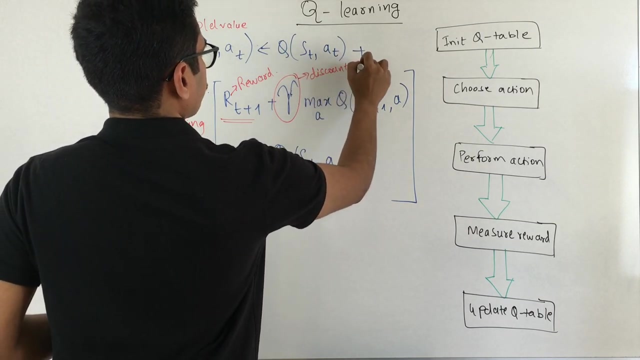 of time, So that is unit increment in time. So that means t plus 1, then accordingly have t plus 2, t plus 3 and so on. This thing we have seen many times, but we have not discussed about this thing. So this is called as a discount or a discount factor. 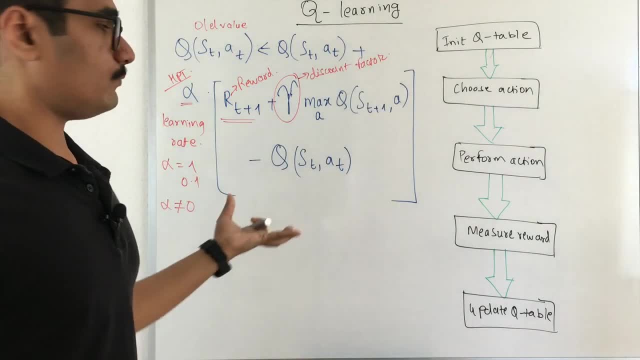 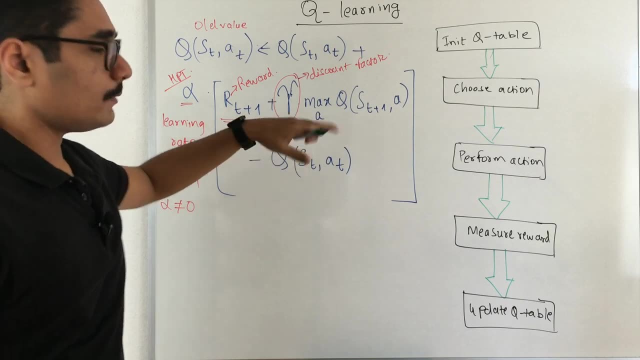 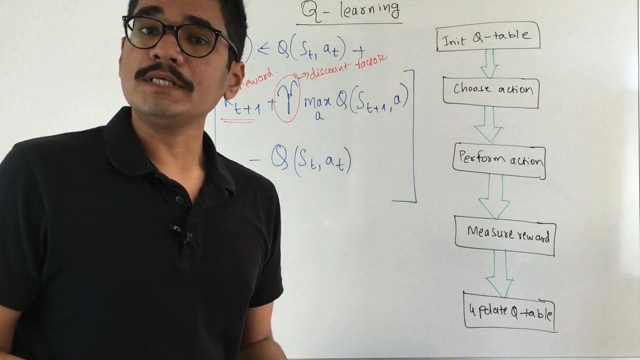 This is also a hyper parameter that you have to tune or you have to put, so discount is done in order to give some kind of balance to this equation, so that it will not jump out of the range or jump out of the expectation. So you multiply with this. 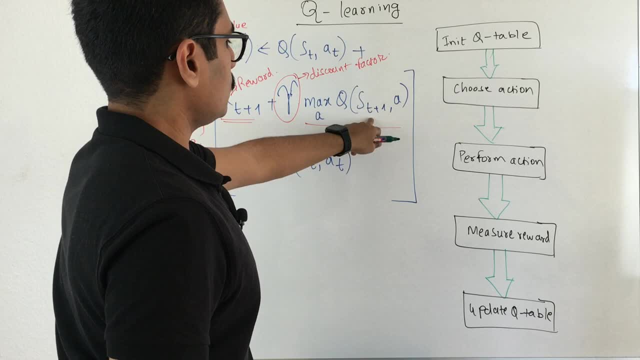 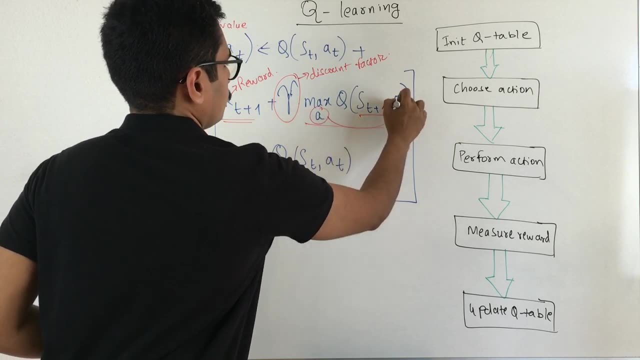 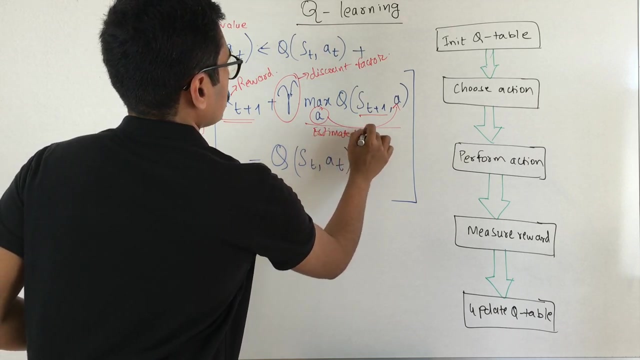 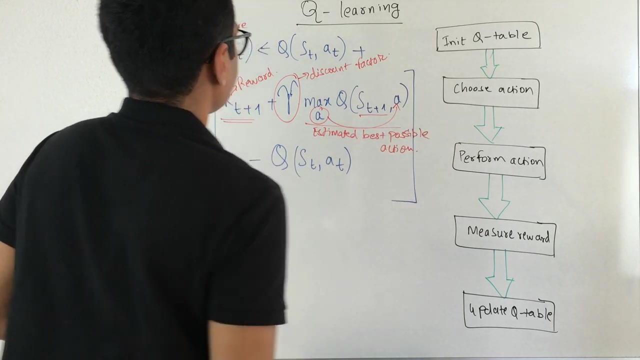 That is the maximum of Q with the next state for the action. So you have to maximize this a which you have here. So that means the best possible action, that is estimated best possible action. So these three things, that is, the reward, the discount factor and the estimated reward. 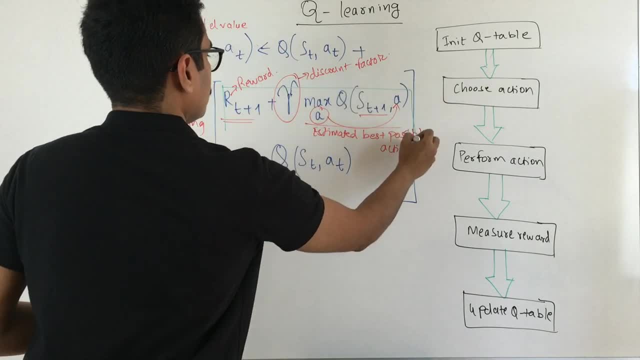 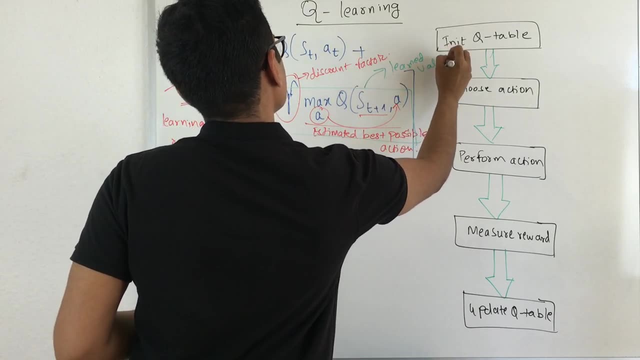 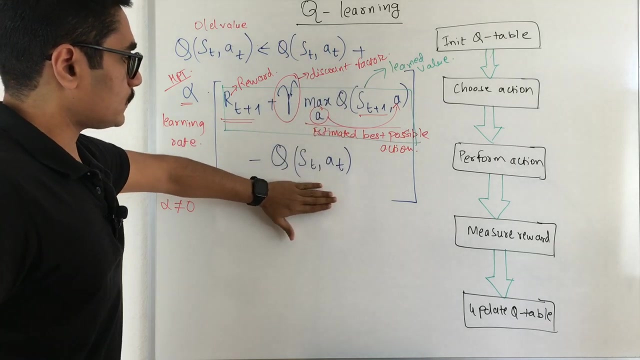 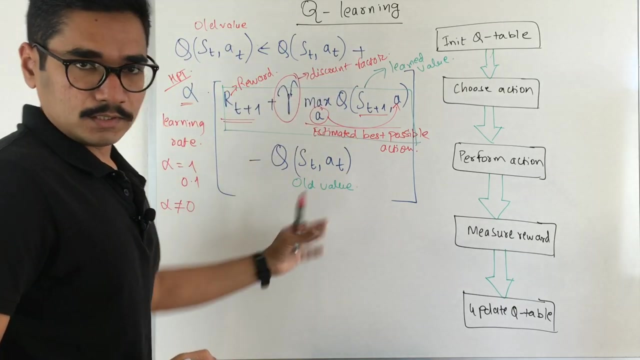 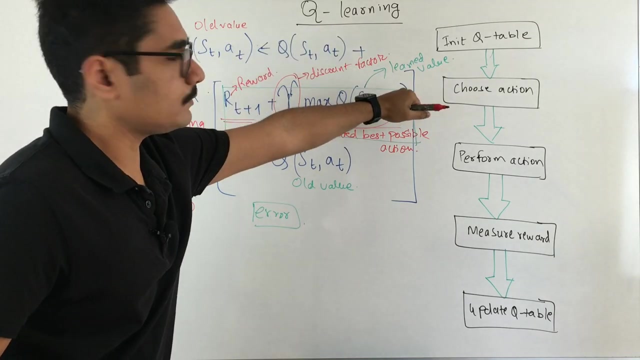 So the estimated best possible action- these three things- comprises your learned value, Okay, and then, once you have this quantity, you do the math here. you subtract that with the old value, So the resultant which you get, that is the error. Okay, So this is the learned value, that is the target value, and this is the old value, that is the. 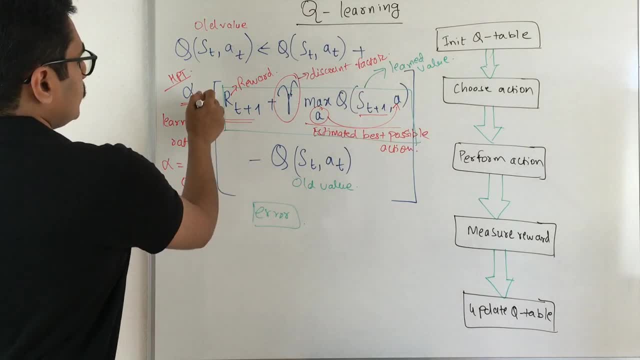 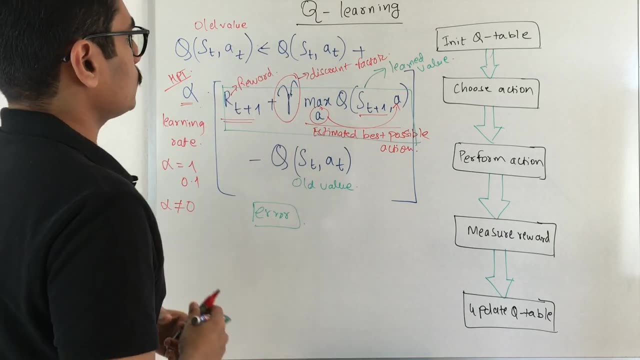 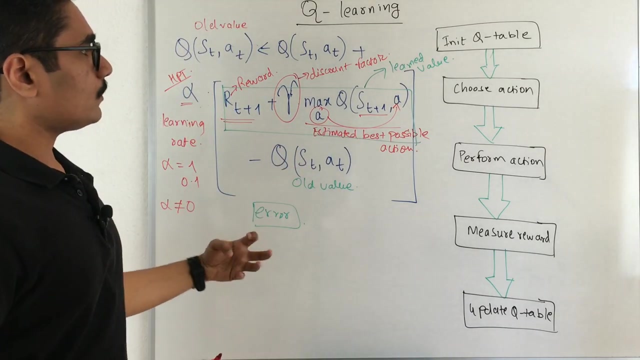 prediction, you get the error. that error you multiply with this alpha, that is the learning rate, in order to correct this so that you can take the best possible action. So this is the algorithm or math behind the Q learning algorithm: how it updates. now, if you want to have a implementation of this, will do a python implementation of the Q learning. 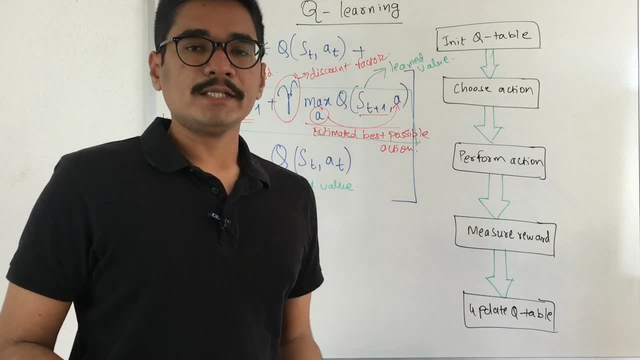 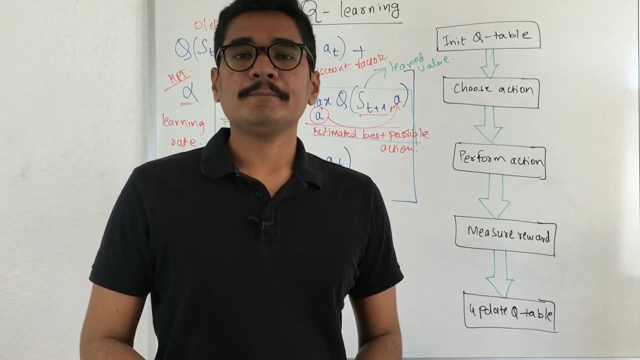 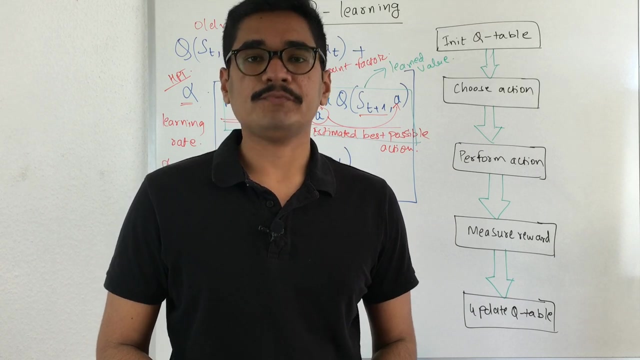 I will make that video to make more understand of this concept. So well, that was all regarding the Q learning algorithm in machine learning- reinforcement learning. so hope you guys enjoyed this video. if you find you got educated what this video please do like, share, comment and if you're new to this channel, please consider subscribing. Thank you very much for watching this video.